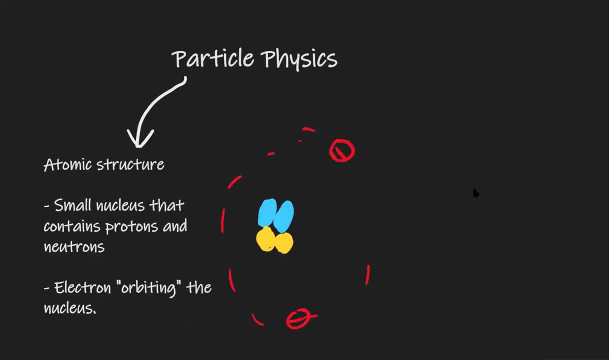 Let's revise particle physics. This video will be following the AQA physics specification. So starting off with atomic structure, The basic structure of an atom is that it has a small nucleus located in the center and that contains some protons and some neutrons. We have electrons. 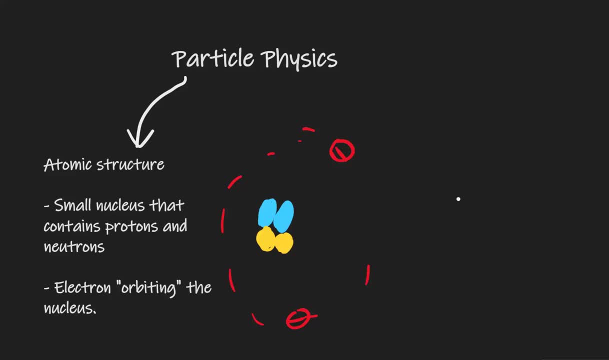 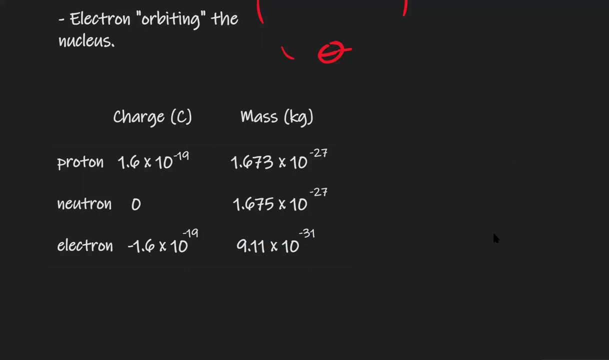 which are sort of orbiting the nucleus around here. In reality they're following this amazing probability density cloud, but more on that later. in quantum mechanics, Most of the stable visible matter in the universe is made out of these particles and they have separate properties. 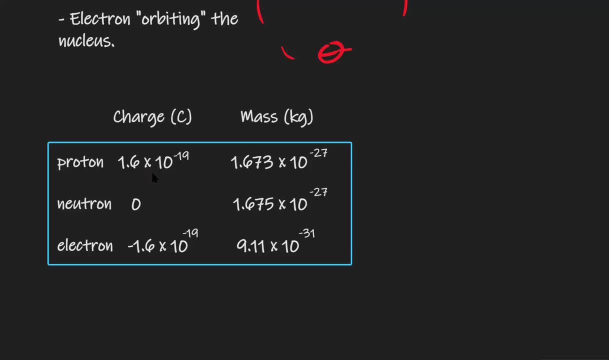 For instance, the proton has a charge of plus 1.6 times the power of minus 19.. The neutron has no charge and the electron has a charge of minus 1.6 times the power of minus 19 pounds. You can see the masses of the particles as well. here We can see that the neutron is just 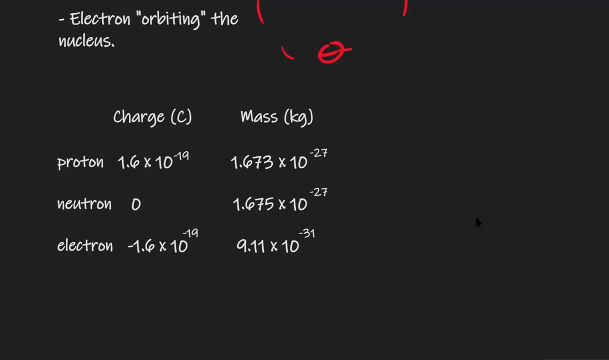 slightly heavier than the proton. Actually, in an exam typically they might be given just up to three significant figures If that's the case. but the proton and the neutron have a mass of around 1.67 times the power of minus 27 kg. The electron has a much lower mass of around 9.11 times. 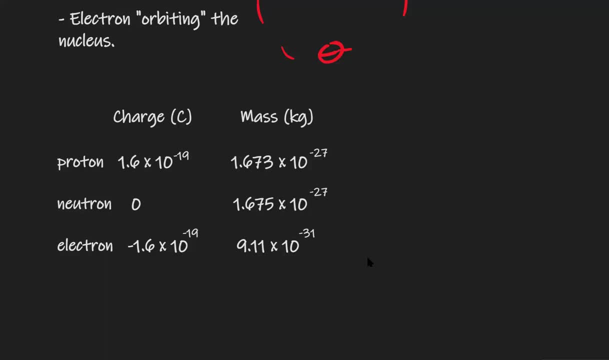 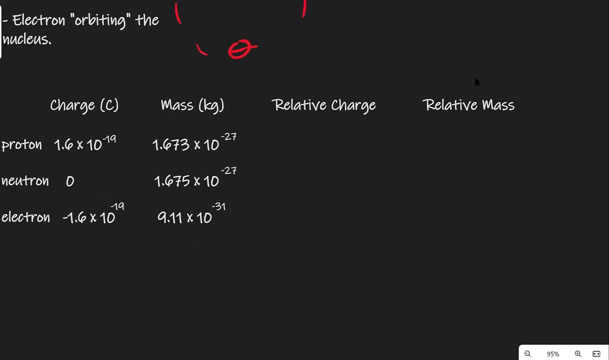 the power of minus 31.. We're going to be using those in physics quite a lot, so we'll probably end up remembering those values. You may also come across a notation that talks about the relative charge and the relative mass In those units. the proton will have a relative charge of plus 1, the neutron will have a relative charge of 0, and the electron a relative charge of minus 1.. 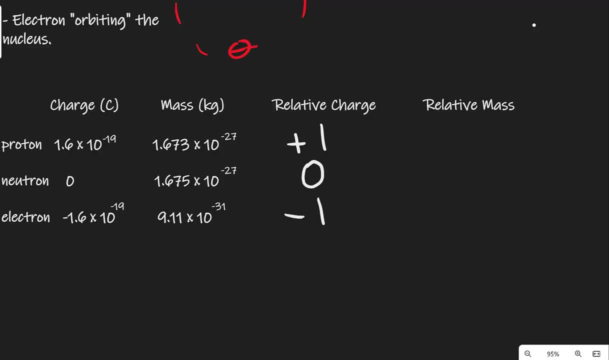 We could also talk about relative mass. In this case, both the proton and neutron are going to have a relative mass of 1, because they have roughly the same mass. The electron, though, is multiple times smaller, and its relative mass is tiny. It's about 0 point, and then three zeros have been 0, 0, 0, 5.. 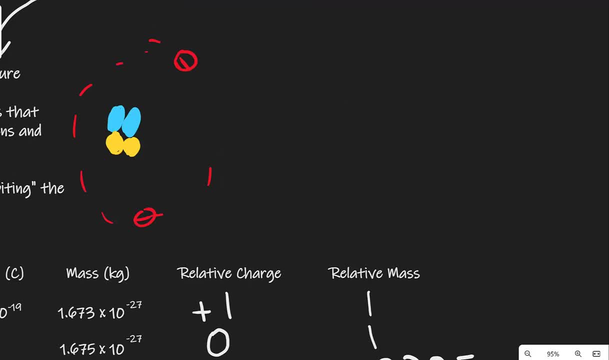 So how can we express this with symbols? Well, imagine that we have some sort of an element. Let's call that X. This element will have a certain number of protons, and we typically write these in this corner over here. The proton number is often given the symbol Z. 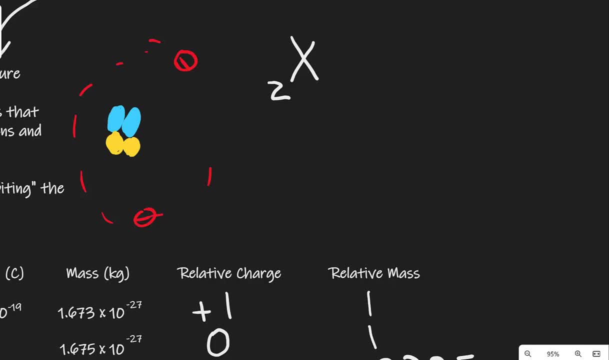 There's also the total nucleon number, which is given the symbol A, and we typically write this down right over here. So let me give you an example. Let's pick helium, for instance. So this over here is my artistic drawing. 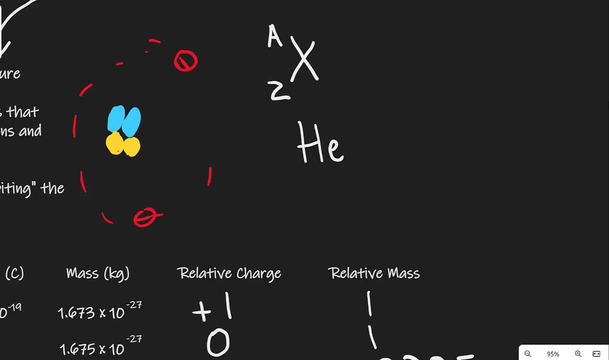 Of a helium atom. the number of protons in a helium nucleus is well 2, so this number here will be 2, because there are two neutrons as well. the total nucleon number A is the number of protons plus the number of neutrons, so this here is going to be just 4.. 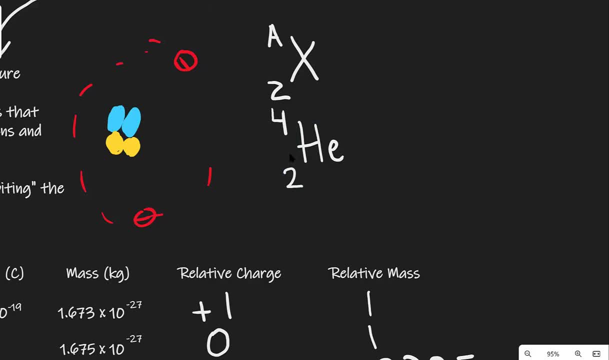 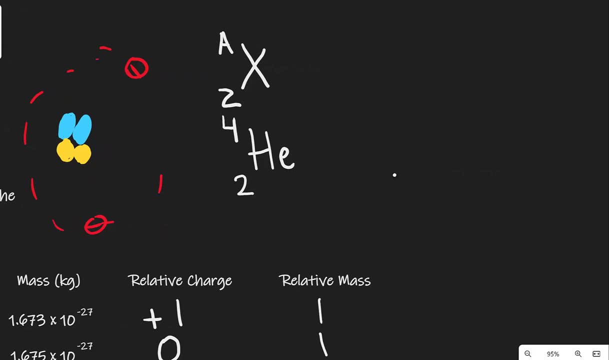 It's important to define that. this number here, the proton number, is the number of protons. The proton number actually defines a chemical element. Let me give you an example. So let's say that we have hydrogen. Let's say we have hydrogen 1, 1,, which is just one proton. 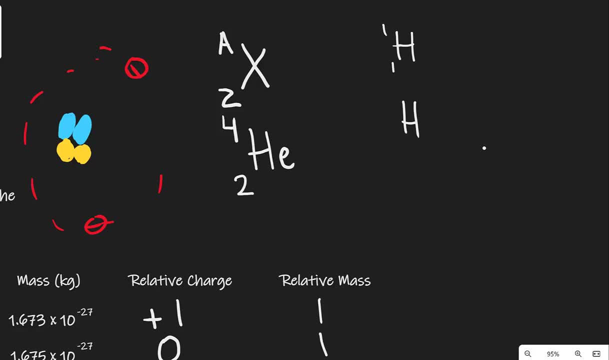 We could also have deuterium, which is still hydrogen. It has one proton, but it also has a neutron, So in the nucleus. so let's say that this is the nucleus of hydrogen 1.. The nucleus of hydrogen 2.. 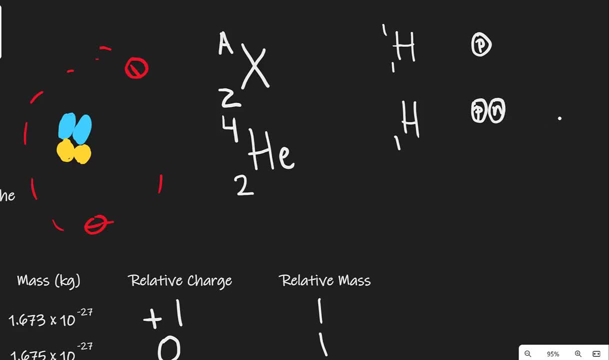 2 will just be a proton and a neutron. This number here is the total nucleon number, which was now going to be 2, because there's two particles in the nucleus. You could also have hydrogen 3,, which will just be a proton and two neutrons, like so. 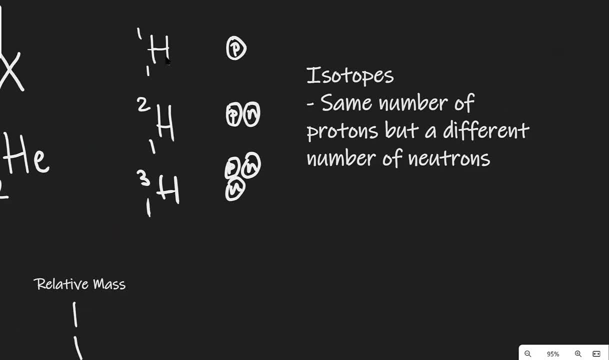 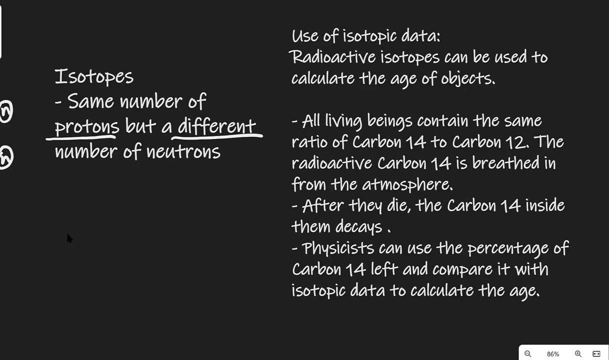 This is known as tritium, And those particles right here are actually examples of isotopes. So an isotope will have this Same number of protons but a different number of neutrons. Isotopes have a lot of applications. 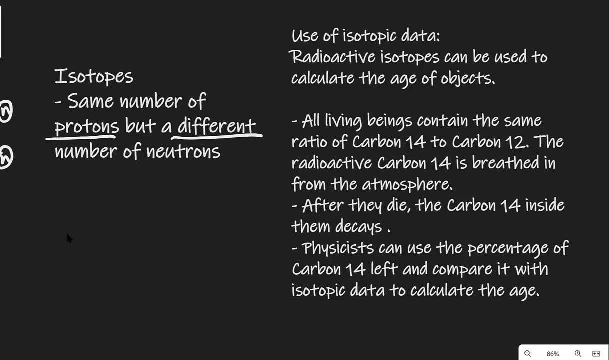 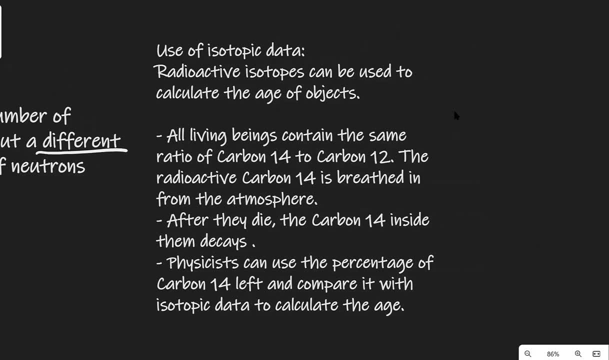 They're used in medicine. They're also used in radioactive carbon dating, which I'm sure you've heard about, And let's use that as an example of a use of isotopic data, which is part of the AQA spec. So, for instance, radioactive isotopes can be used to calculate the age of objects. 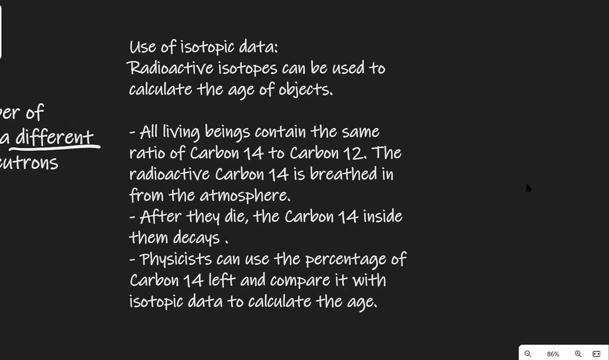 Now how does that work? So all living things, or all living beings, contain the same ratio of carbon-14 to carbon-12.. Now carbon-14 is actually radioactive and we're actually breathing some radioactive carbon-14 from the atmosphere. 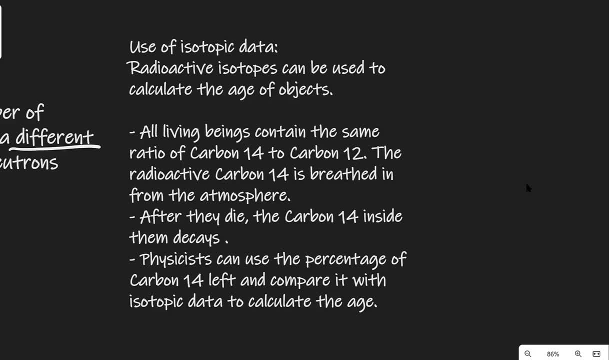 How is that produced? It's produced by cosmic rays, which essentially strike the atmosphere of the Earth. Imagine that this here is the Earth And this is the Earth, And they can cause some reactions, which means that over here we can have some carbon-14 that's been created after interactions with a cosmic ray. 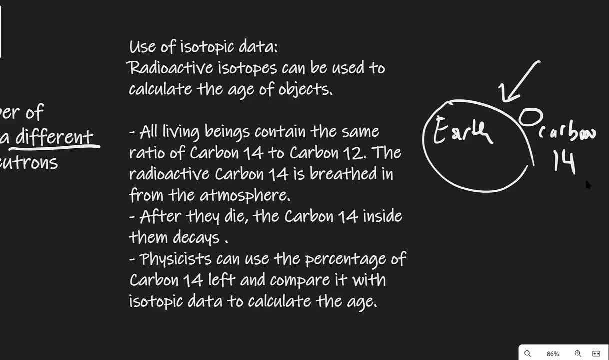 This diagram is obviously not up to scale. by the way, Now we actually have a constant ratio of carbon-14 to carbon-12 in our bodies, And after an organism dies, for instance a tree, the carbon-14.. Well, the ratio of carbon-14 to carbon-12.. 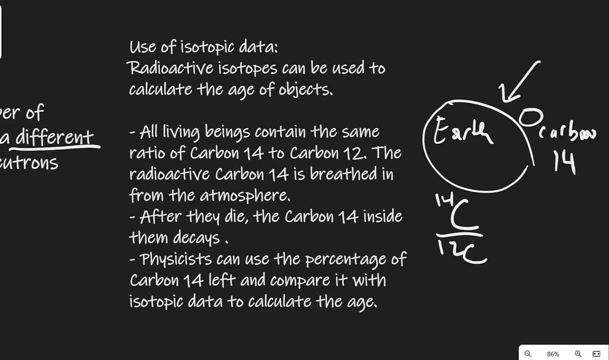 Well, the ratio of carbon-14 to carbon-12 starts to decrease. Now physicists can use the percentage of carbon-14 left and compare it with isotopic data- a really important word to actually calculate the age. There's another formula that we should know, and that is the specific charge. 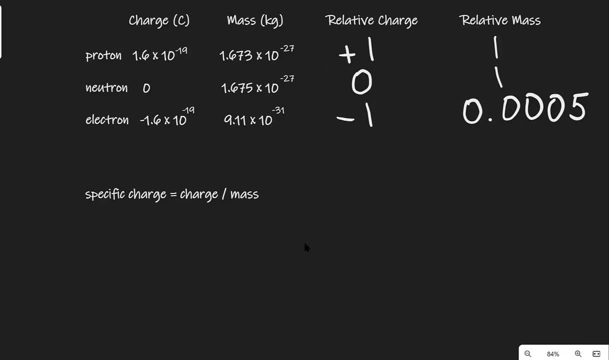 This is just the ratio of the charge of a particle divided by its mass. We can also see from this formula that the specific charge will just be measured in units of coulombs per kilogram. If we're dividing by mass or by kilograms, we often write this as kg to the power of minus one. 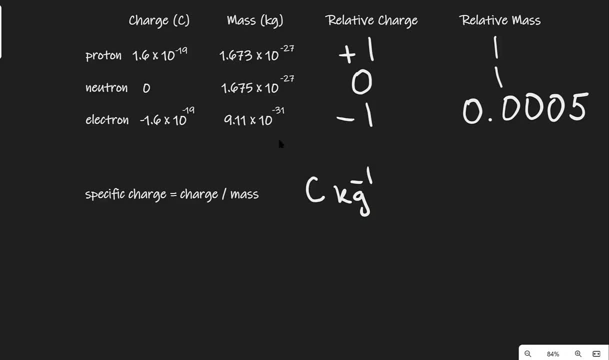 Well, let's do a little bit of an example. Let's pick a particle. So should we just start off with the proton? And what is the specific charge of the proton? Well, in order to find that, for the proton, this will be equal to its charge, which is 1.6 times 10, to the power of minus 19 coulombs. 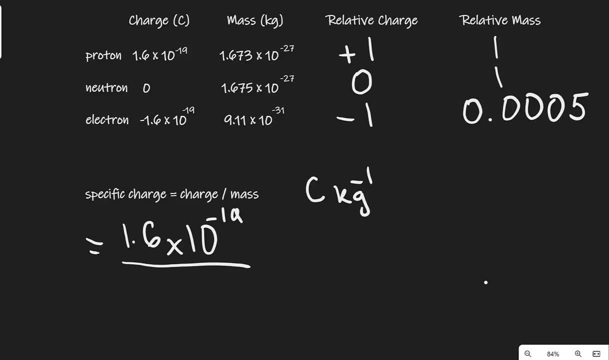 And we're going to be dividing that by the mass, That by the mass of a proton. So we'll just use 1.67 times 10 to the power of minus 27.. Let's put this into a calculator And up to, let's say, three significant figures, or let's use two. 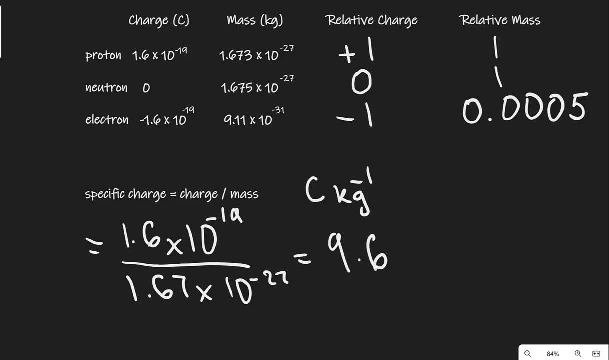 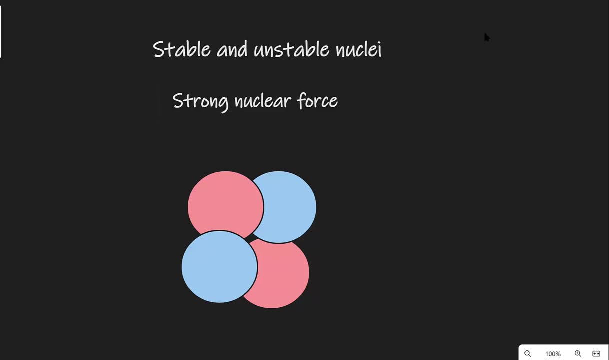 We're going to get around 9.6 multiplied by 10, to the power of 7 coulombs per kilogram. Now let's see what makes nuclei stable or unstable. In order to do so, we need to think about what are the forces inside of a nucleus. 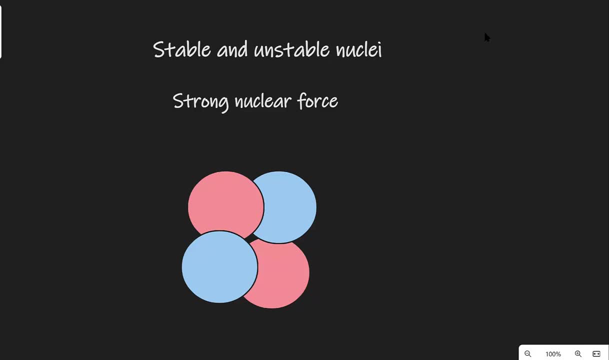 And ultimately we need to discuss the strong nuclear force. So imagine that this over here is just a nucleus. So the red particles are protons, These blue particles, let's say, are neutrons. So what forces are acting on the nucleus? 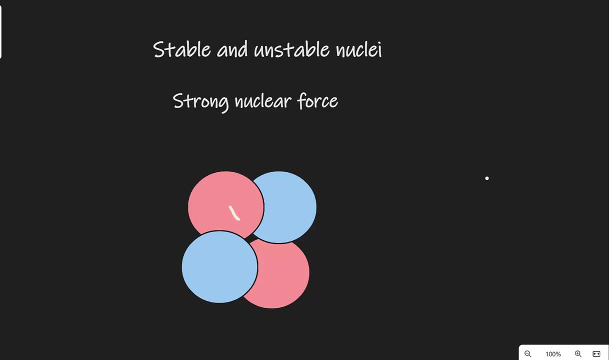 First of all, we have the force of gravity, Which is trying to pull us out of the nucleus. Pull all these particles together. This is actually very weak, as we're about to discover in this course. So Fg will be pointing somewhere, towards the center of mass. 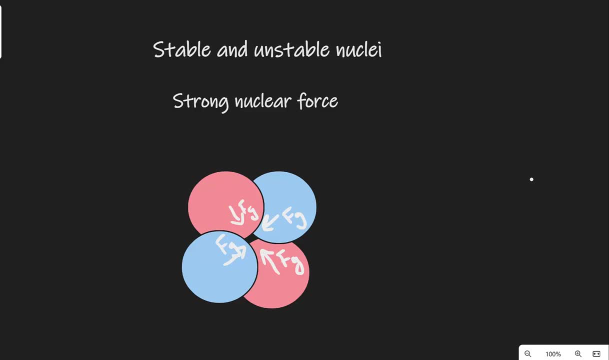 Now there's going to be another force acting between the charged particles And remember, because the protons are positive, two positive particles will repel. So there's going to be another force And this will be the electrostatic force of. 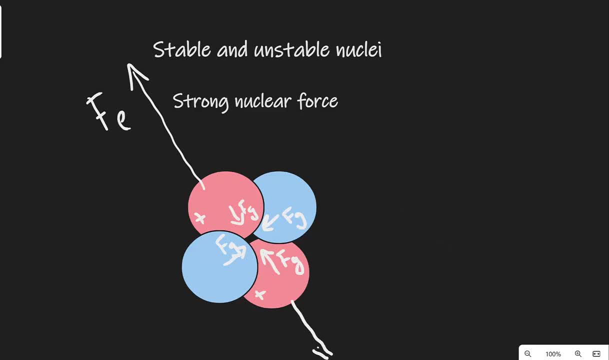 Repulsion, Which will be very, very large indeed, So much that it can't actually draw this vector out properly. Now, if those were the only two forces to exist, This means that matter would just separate out And this particle would just fly out. 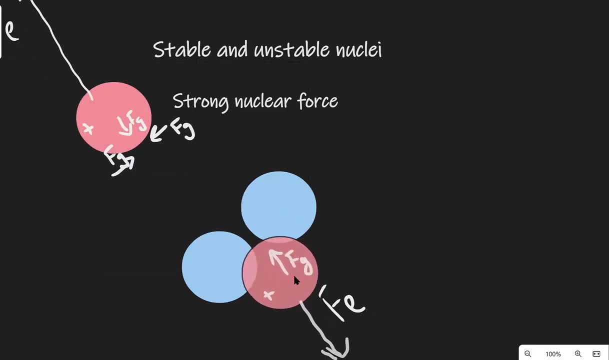 And this particle here would also fly out, Because they are repelling each other. Now they don't, Which means that there needs to be another force that exists within the nucleus That is gluing the nucleus together. And well, this force is the strong force that is responsible for bringing and gluing in the nucleus together. 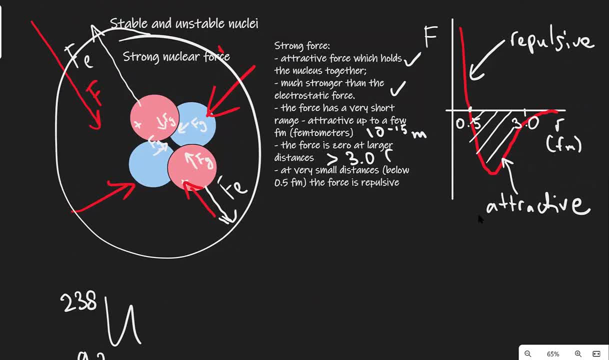 Now, interestingly, if the size of the nucleus goes beyond the 3 femtometers, We're very likely to receive a decay particle. To see a decay particle? This is because the strong nuclear force can only act within this region. So look at that. 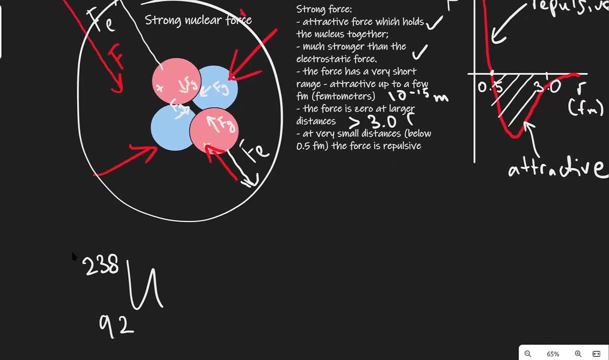 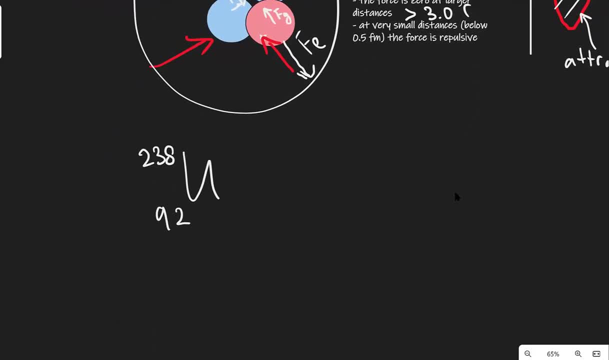 At the moment I've only drawn 4 particles, But what if we had 238 particles? This is one classic alpha decay of uranium-238.. So this will actually emit an alpha particle And it will decay to Thorium. 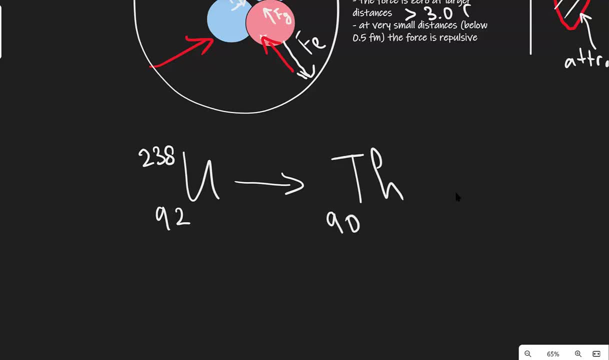 So thorium will be element 19.. Because it's losing an alpha particle, Which The alpha particle is just 24.. This means that our nuclear number is going to be 238.. Take away 4., Which is going to be 234.. 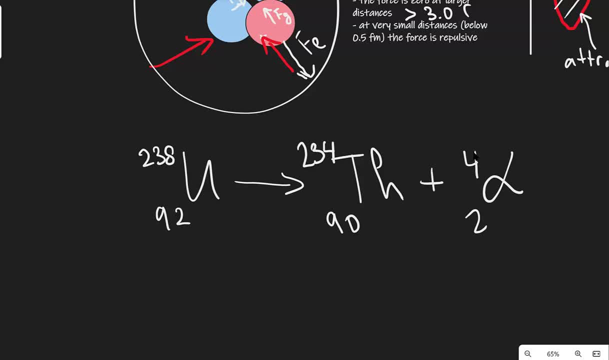 And this right here is an example of an alpha decay equation. We're emitting an alpha particle And we have a conservation of all the numbers. Our proton number is conserved, So 92 is equal to 90 plus 2.. And our nucleon number is conserved. 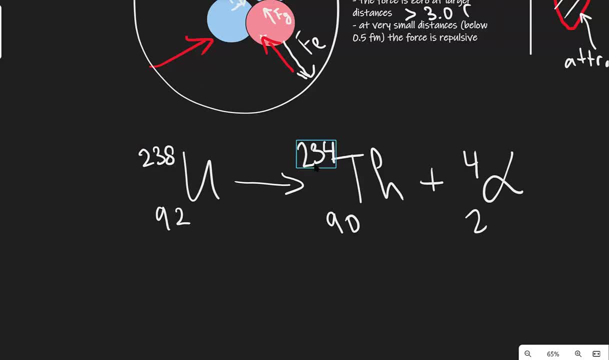 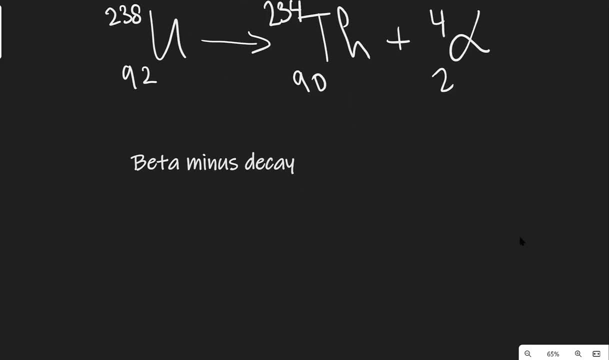 So 238 is equal to 234 plus 4.. Particles can also decay via beta minus decay. So this one here was alpha. Let's see what beta is. So in order to do so, Let's have a look at the decay. 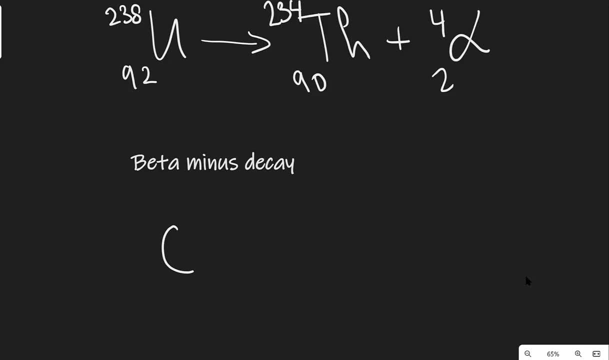 Let's say carbon 14.. So carbon 14, as we said, That is radioactive And it's carbon 614.. Now this actually decays to nitrogen, Which is Has a proton number of 7. And a nucleon number of 14.. 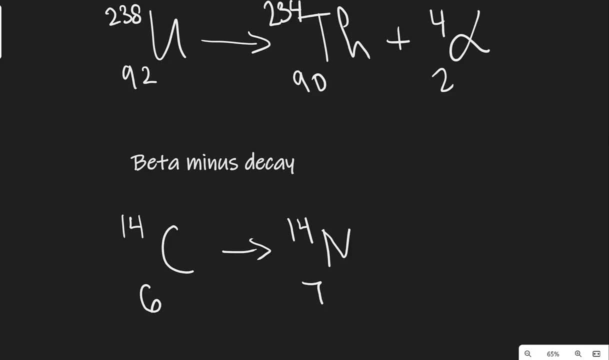 In order to do so, We need to keep all the numbers, All the fundamental numbers, in this equation clear. So, for instance, The charge, The relative charge, here is plus 6.. On the left hand side, However, on the right hand side, is plus 7.. 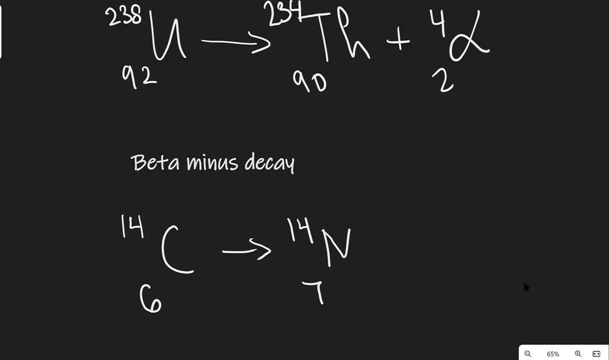 So the only way we can do that Is if we have a beta particle come out as well, And this beta particle is actually a simple electron Which has a relative charge of minus 1. Nucleon number of 0. Now our equation is balanced. 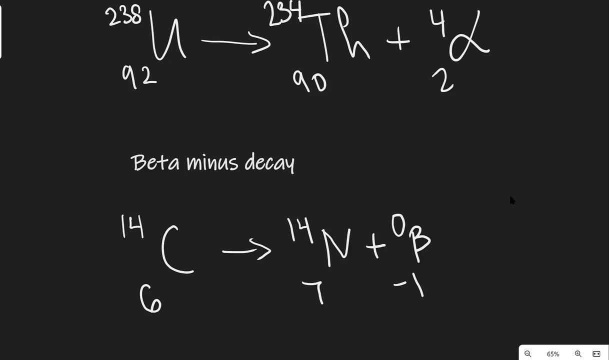 Now this is an example of beta decay. However, this is not complete. Experiments showed that the energies, Or the total mass energy, on the left hand side Was not equal to the total mass energy on the right hand side, So scientists hypothesized. 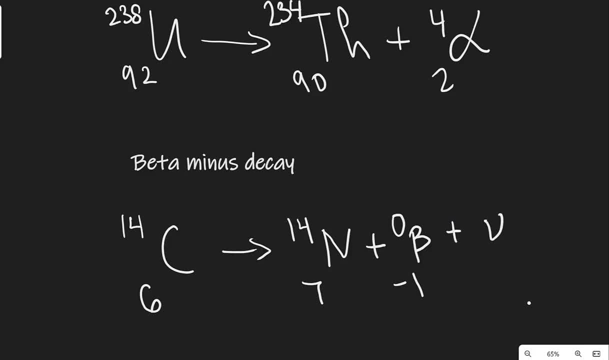 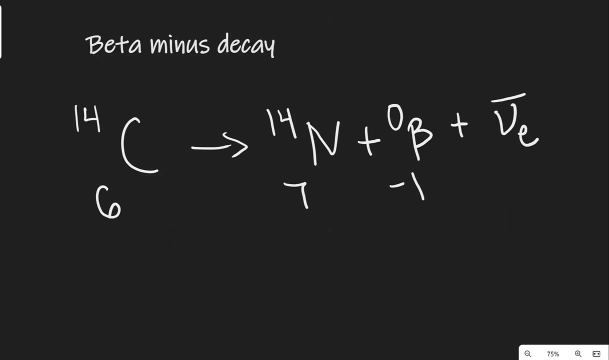 Another set of particles called a neutrino, Known as the electron neutrino actually, And this is actually an anti-particle In this reaction That must occur, And this is an example of a beta minus decay equation. Have a look at something incredible. 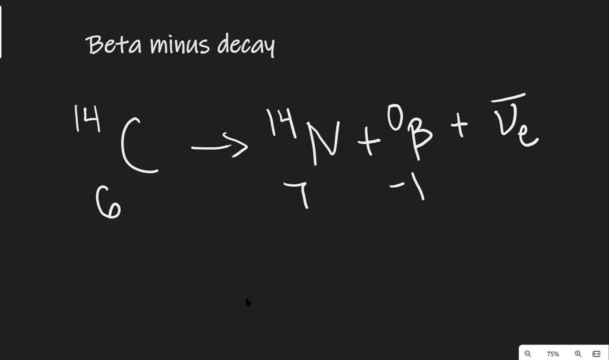 The total number of protons here is 6. Whereas the total number of protons here is actually 7.. So by the power of something called the weak nuclear force In beta minus decay A neutron has turned into a proton. So an actual neutron turns into a proton. 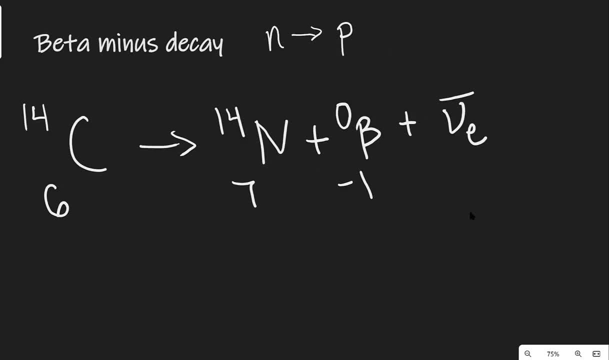 A couple of tips to remember. Every time we have a beta minus decay equation, Obviously we get the beta particle, Which is just an electron. The nucleon number will always remain the same Because a neutron will turn into a proton, Meaning that this number here is constant. 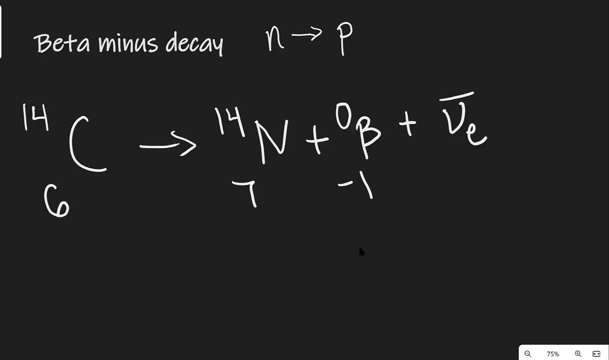 And this number, The proton number, will always go up by 1.. We're also going to get the anti-neutrino. I'm going to be talking about anti-particles next. Have a good rule of thumb to remember Is that, if you can see this dash here for the minus sign, 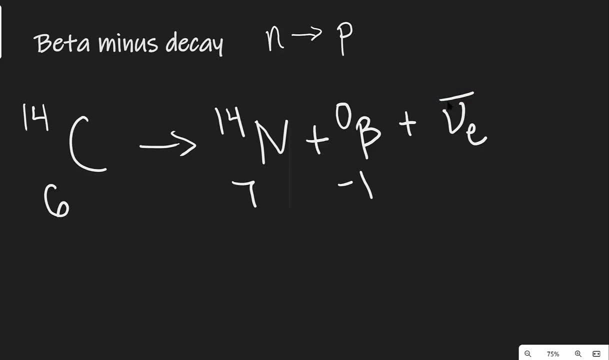 You can definitely see an anti-particle. An anti-particle is signified by this dash at the top of the particle. So in physics, Each fundamental particle has its own anti-particle. How amazing and incredible is that. For instance: 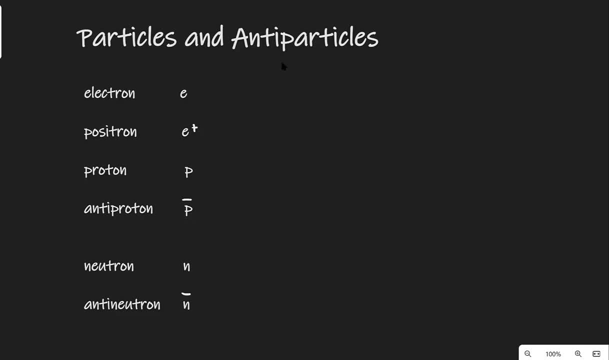 The electron has its anti-particle, Being the positron. The proton has its twin anti-particle, Which is the anti-proton, The neutron and the anti-neutron, So on and so forth. Now, how do the properties differ? 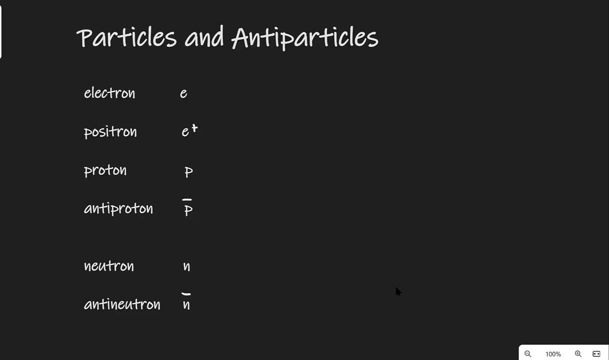 First of all, The mass is exactly the same. So, for instance, Both the electron and the positron Have a mass of 9.11 times 10, to the power of minus 31 kg, And the positron also has a mass of 9.11 times 10, to the power of minus 31 kg. 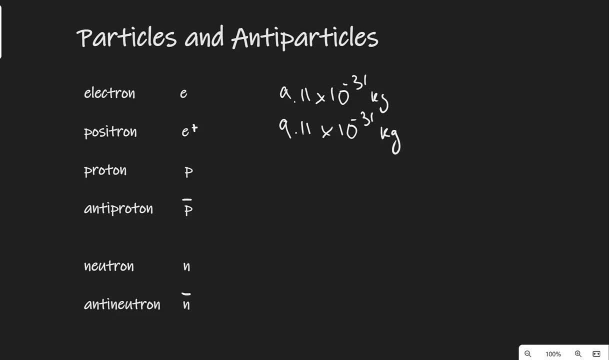 And this is where things start to get really interesting. The electron has a charge of minus 1.6 times 10 to the power of minus 19 coulombs, But the positron has a charge of plus 1.6 times 10 to the power of minus 19 coulombs. 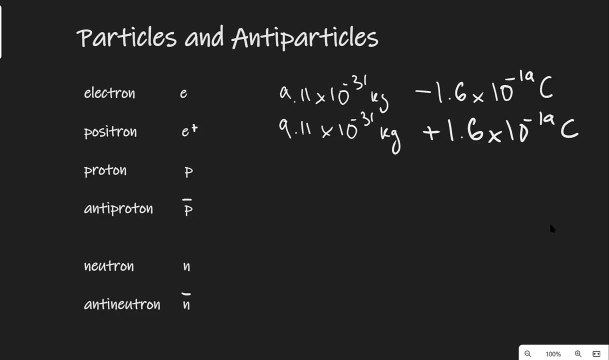 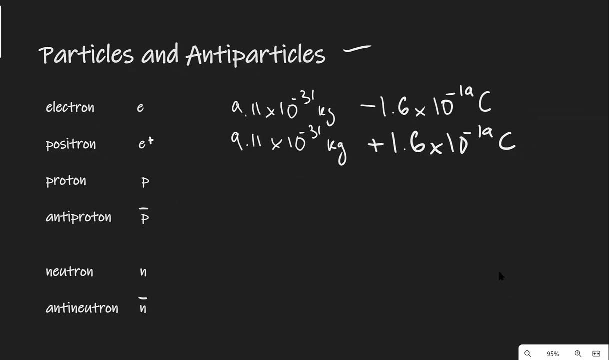 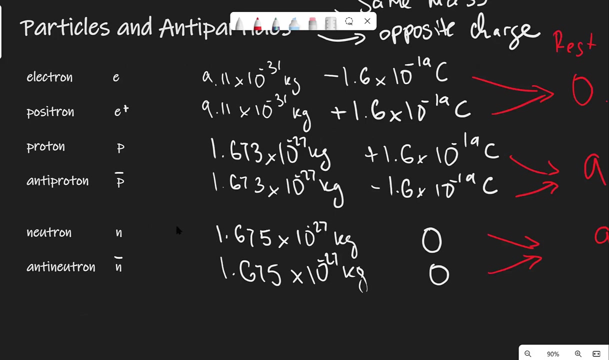 So, in short, Each anti-particle has the same mass, And let's write this down over here. So anti-particles have the exact same mass, They are the same particle, But they have the opposite charge. Let's compare the properties of the other particles. 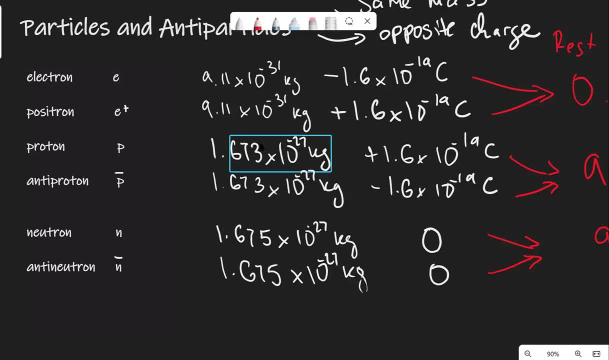 So, for instance, The proton and the anti-proton: They have the exactly same mass, As I said, with the opposite charges. So plus 1.6 times 10 to the power of minus 19.. And minus 1.6 times 10 to the power of minus 19.. 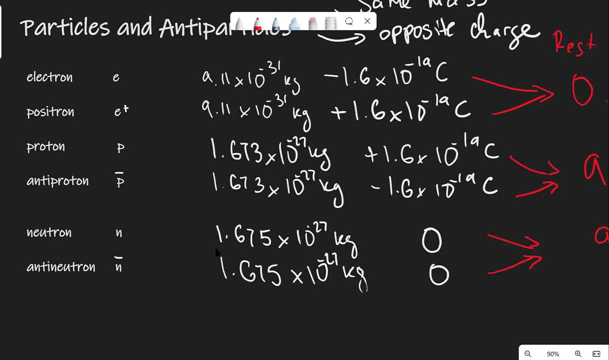 The neutron and the anti-neutron. So they have the same mass: 1.675.. Tiny bit larger than the proton. And they actually have the same charge, Because the neutron has zero overall charge And the anti-neutron has, once again, a zero net charge. 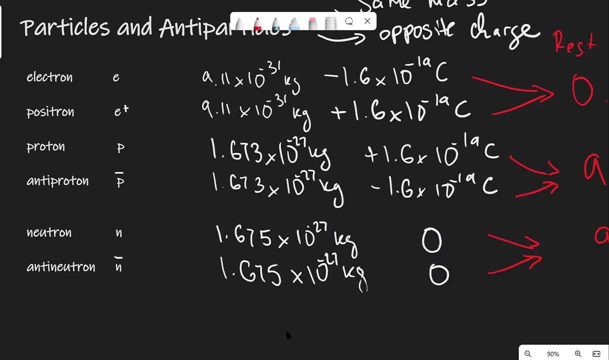 People often ask me: Why are those two particles different? The answer to this will be apparent once we start doing quarks. They are actually a different particle. They are made out of anti-quarks instead of quarks, And it just turns out that the properties are such that the net charge is zero. 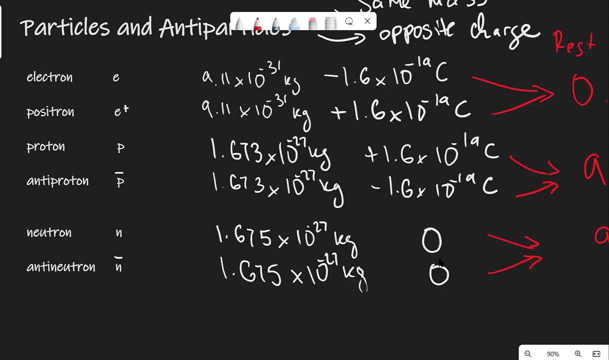 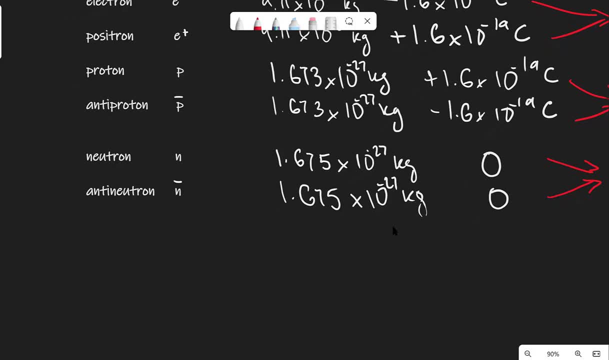 They also have an opposite spin, Which is another property that we don't really do much of during A-level. We actually need to know about one more particle in our exam, And this is, of course, The neutrino, So let's just write this down as the neutrino. 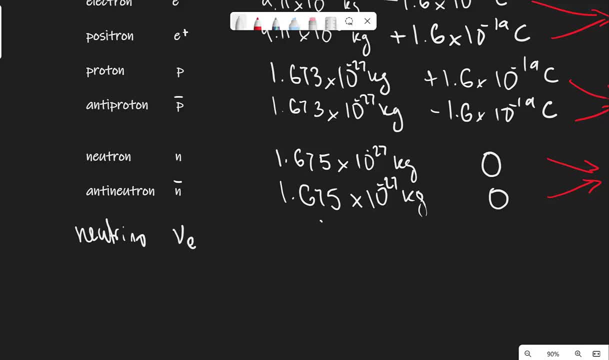 And the symbol for an electron neutrino is just this: It has a tiny, tiny mass. It's very, very close to zero. It is just above zero. It's not actually massless, though, So I'm not actually going to write zero. 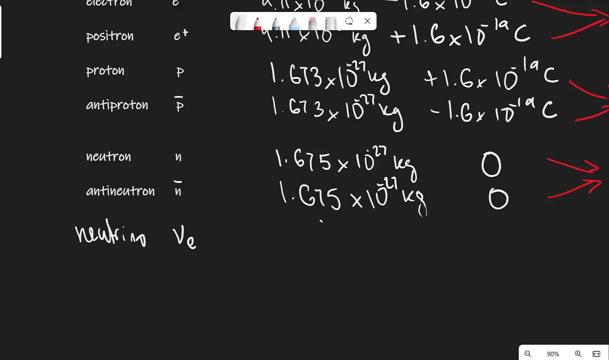 Loads of textbooks write zero, So we can just say that the mass is basically negligible. Should we just write negligible? And it does have a charge of zero, though? Now, the symbol for the anti-neutrino is such, And it has exactly the same properties. 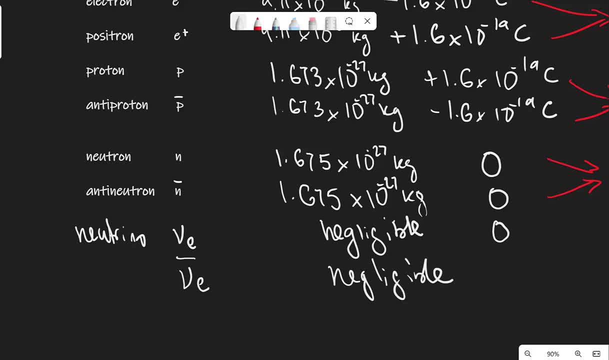 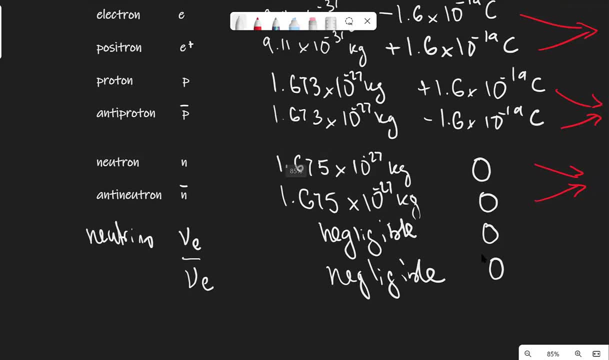 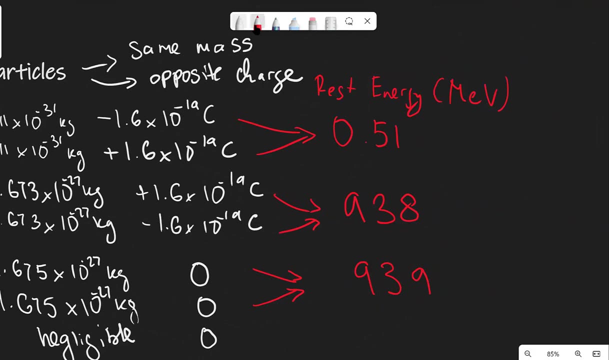 So it has negligible mass And it has a charge of zero. Now let's have a look at another property which is very, very useful for particle physicists, And that is rest energy. That is typically measured in mega electron volts. If you're wondering, where on earth does this unit actually come from? 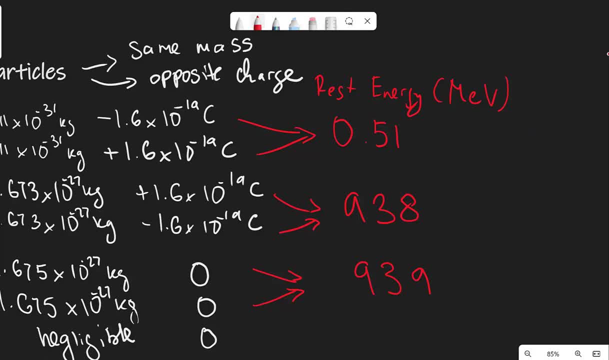 The mega electron volt. We're going to do this later in the course, But basically electrical energy is equal to the amount of charge multiplied by the voltage. So if our voltage is, let's say, the electron, Or if our charge is the electron charge, 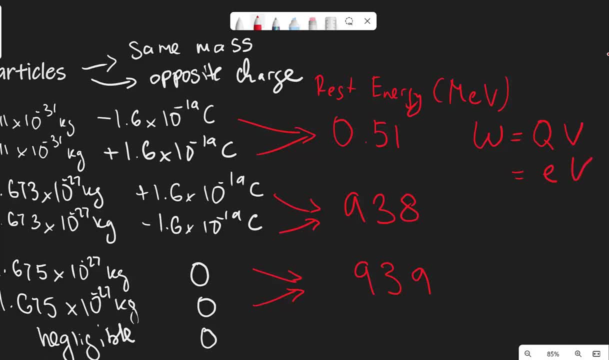 And our voltage is the voltage that we've applied, Let's say a volt. We can get the unit of one electron volt. In this case, a mega electron volt was going to have a factor of ten to the sixth Right over here. 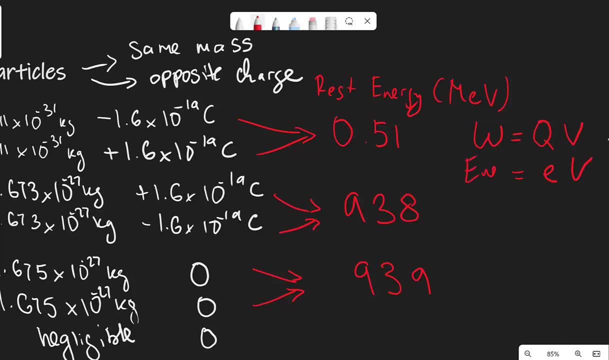 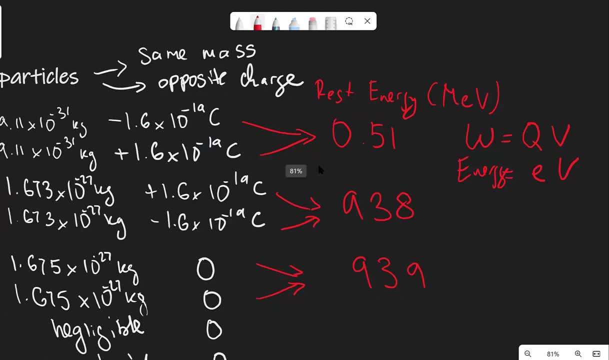 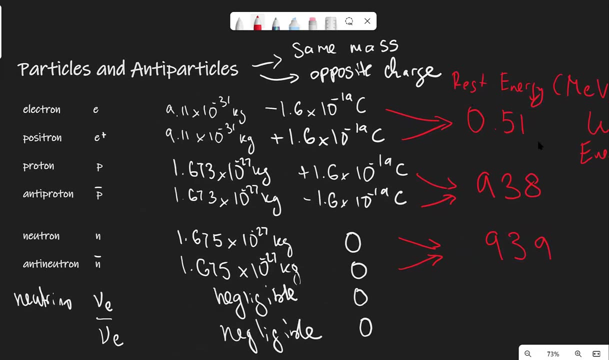 But this is just a unit of energy. So those two particles which are the electron and the positron, Should we just zoom out a little bit- They actually have An energy of A rest energy of 0.51 mega electron volts. 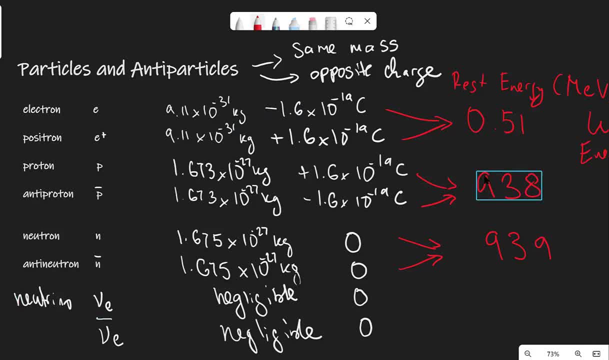 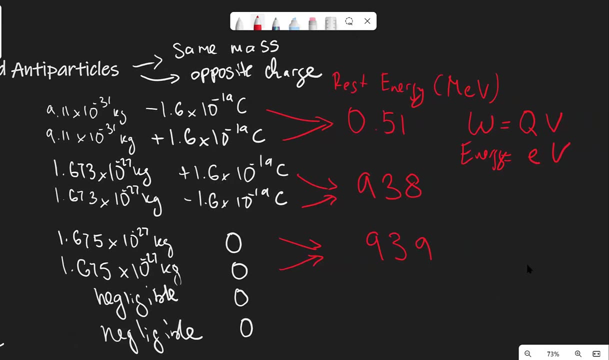 The proton and the anti-proton Around 938.. For the neutron and the anti-neutron It's around 939.. So just a tiny bit higher, Just for comparison. Recently at the Large Hadron Collider- And I'm filming this video in 2022.. 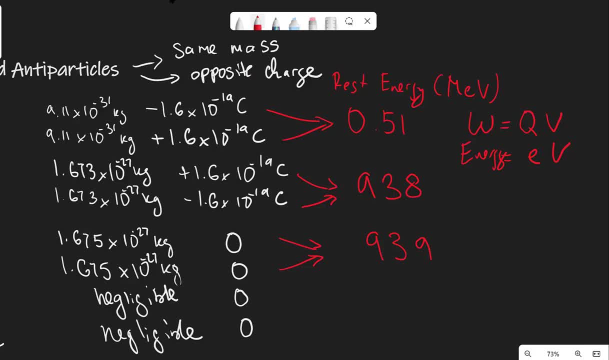 They reached an energy Which was 13.6 tera electron volts And this is the current record, I believe, Unless the OHC has managed to go above that in the last few weeks. But as far as I know it's 13.6 tera electron volts. 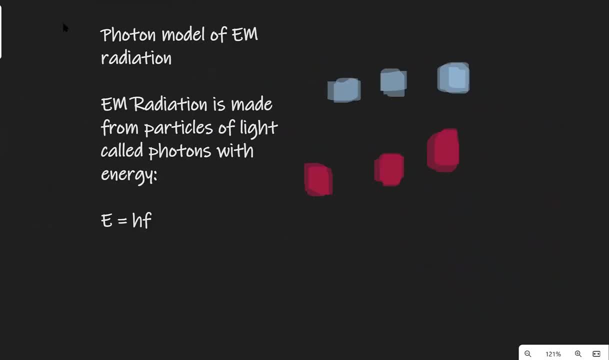 Is the maximum energy that we've smashed particles together. Now, in order to explain the next part of particle physics, We need some understanding of the photon model of EM, Or electromagnetic radiation. Electromagnetic radiation Is actually made from particles of light. 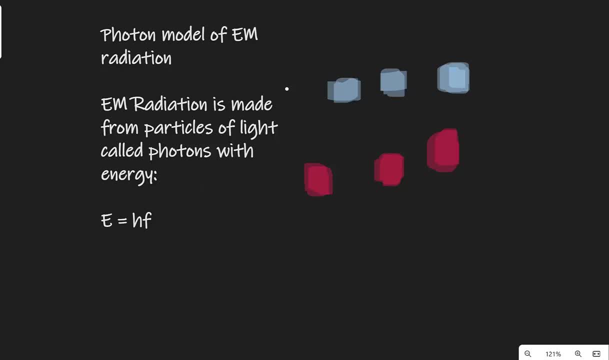 Which are called photons. Now, light has wave-like properties, Such as diffraction, interference etc. But it really is a particle. And each of those fundamental units of photons Have energy, given by the following: The energy is proportional to their frequency. 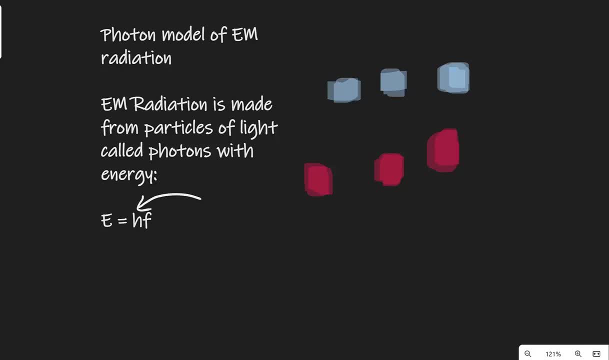 And the constant of proportionality is known as Planck's constant, Which is one of the most fundamental constants That we know of, And the value of Planck's constant Is actually very, very small: 6.63 multiplied by 10 to the power of minus 34 joule seconds. 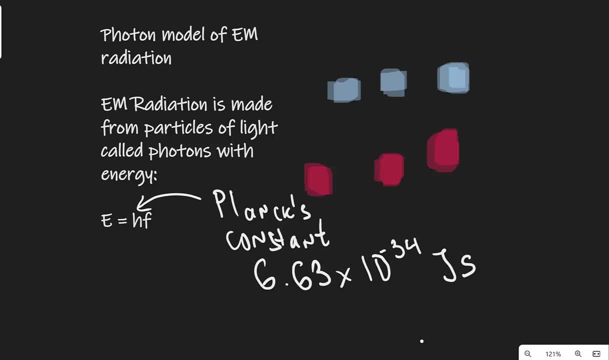 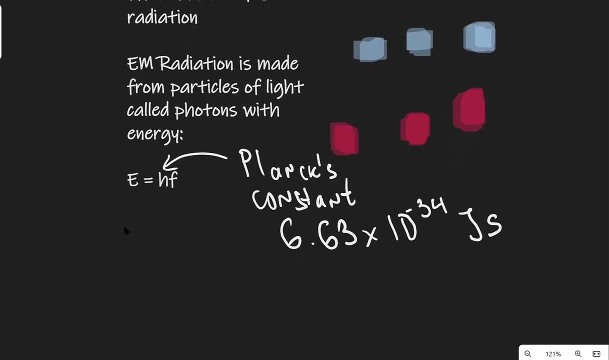 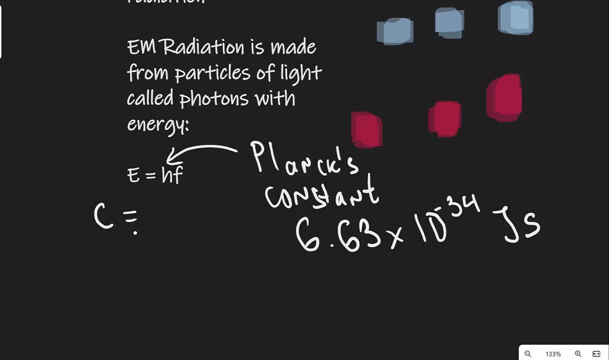 The wave frequency Is linked to the wavelength, Which is given by the wave equation, Which is, of course- Let's just zoom in a little bit- That the speed of light Or any wave-like feature Is given by the frequency Multiplied by the wavelength. 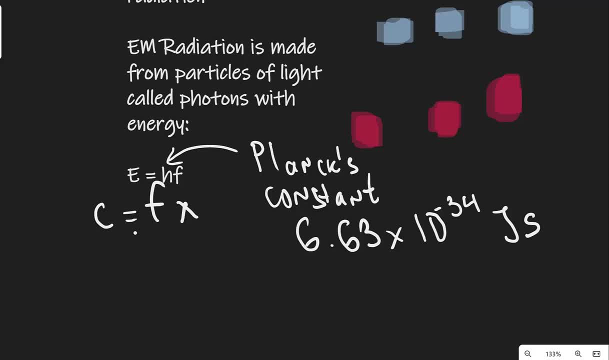 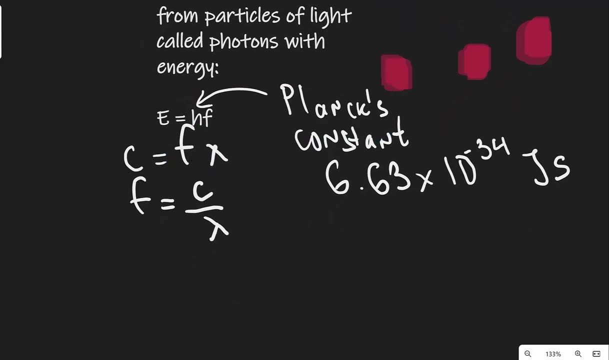 So let's just write the wavelength like that. This of course means that the frequency Is just equal to the speed of light Divided By the wavelength, And we can take this equation And we can sub this into here. We can get our second equation for the energy. 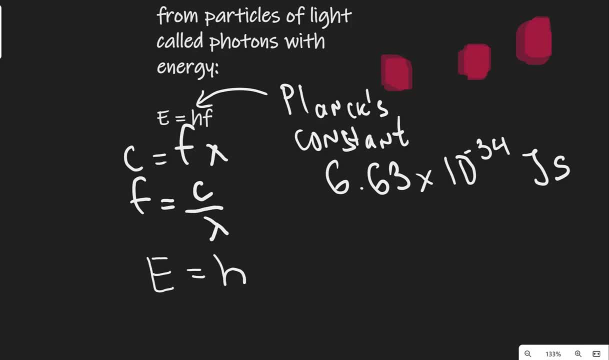 That is, that the energy Is equal to Planck's constant Round the frequency. I'm going to write C over lambda, Just to summarize. We can also write this as: E is equal to HF And this here is the energy of a single particle of light. 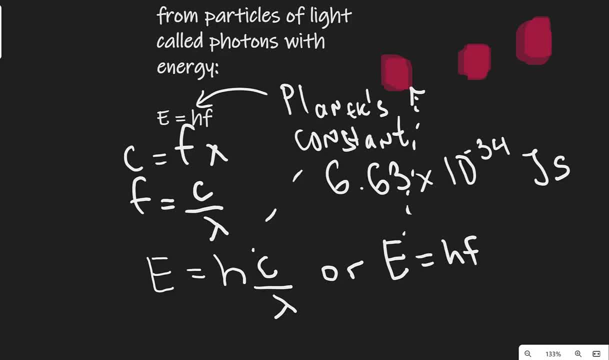 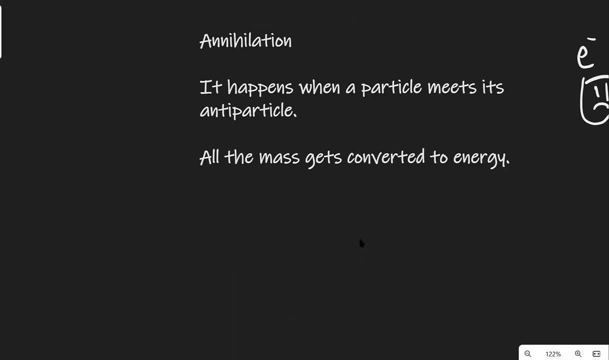 Known as the photon. There are two equations for it. So the reason why we covered the photon theory Is because we want to understand annihilation. So annihilation occurs When an antiparticle meets a particle And all the mass gets converted to energy. 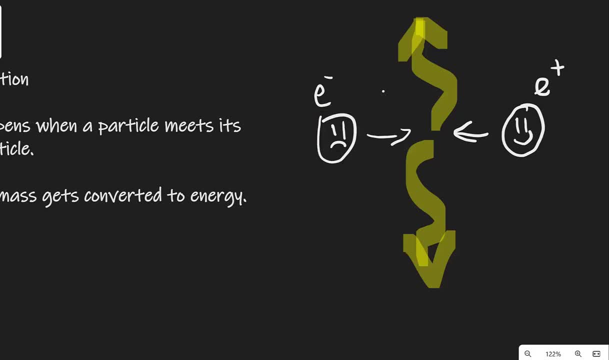 Through this process. Imagine that we have this electron over here That meets a positron. All of their masses are going to get converted To photon energy. So this photon here, That is this coming out, Will have a certain energy. We can call that. 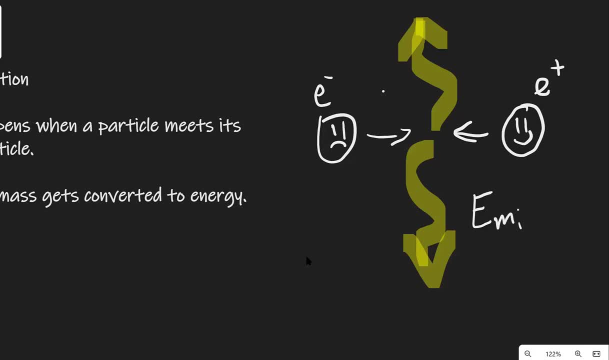 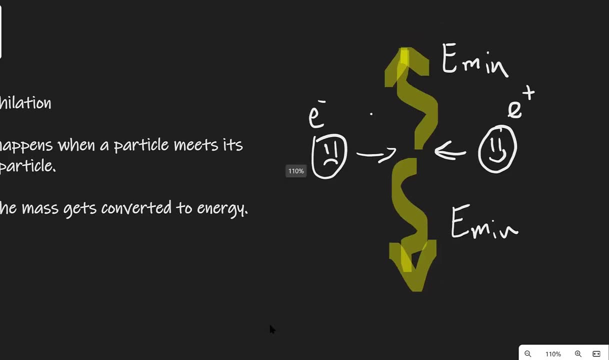 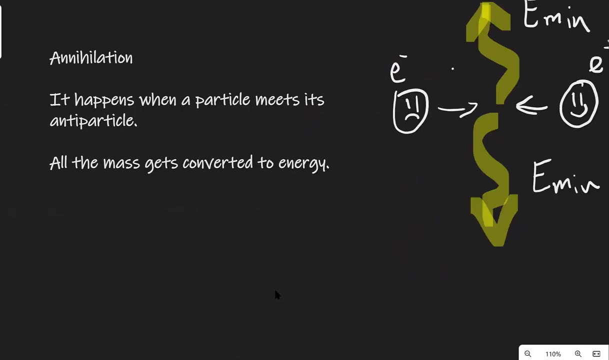 Some sort of a minimum energy. Let's call that E minimum, And this one here Will also have some energy Which is E minimum. We can use energy conservation And actually Estimate the wavelength Of these photons, Because this here was a minimum energy. 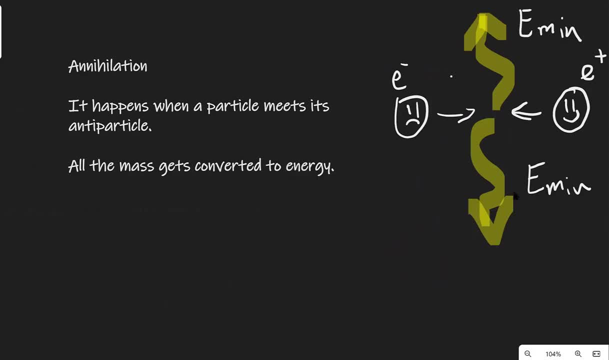 The wavelength will actually be a maximum. So how can we actually calculate The maximum wavelength? Let's call that lambda max. Well, remember Those particles, The electron and the positron, Have some rest energy. Typically, this will be given in the question. 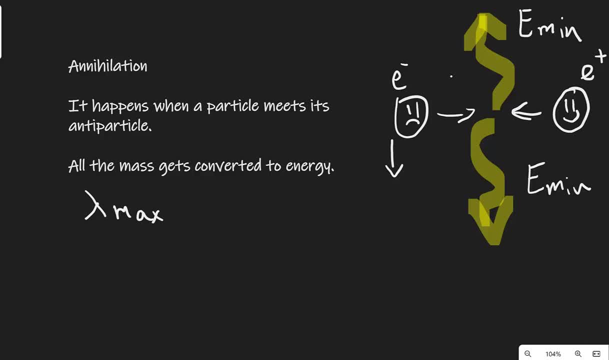 But in the table A few slides ago We mentioned that this was around 0.511 mega electron volts. So this means You can think of this As our input energy And twice that amount, So twice times 0.511.. 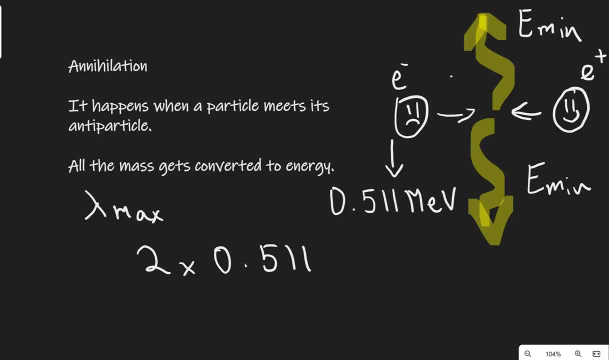 Mega electron volts. Mega is times 10 to the power of 6. And the electron volt Is 1.6. Times 10 to the power of Minus 19.. And this is our input energy. We can set that up. 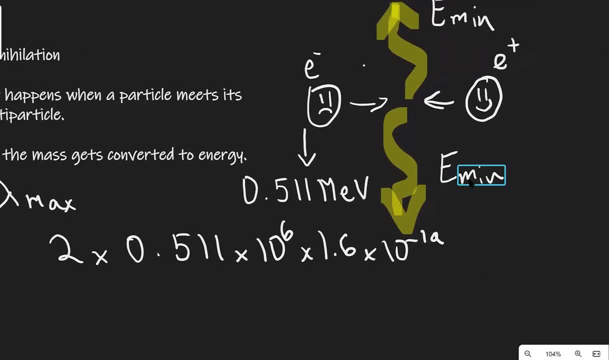 As a minimum. So we can set that equal To the energy afterwards, Which will just be the energy Of the two photons. So we can say that this here Will be equal to twice The energy of a photon. But what is the equation? 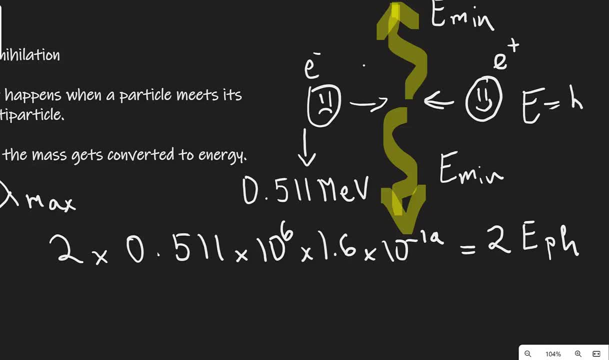 For the energy of a photon. Remember, the energy of a photon Is equal to just Hc over lambda. So rather than energy of a photon, I can literally just write Twice Planck's constant And c is just the speed of light. 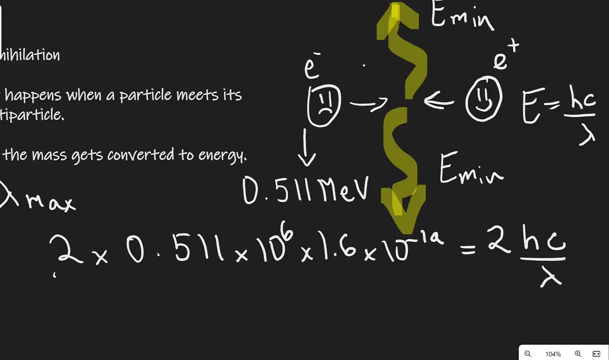 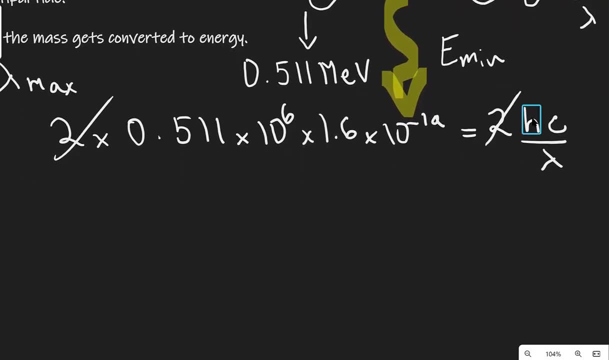 Like. so Now, all I need to do- now I can actually cancel out those tools- Is to rearrange for lambda And then plug in Some values for h and c. I'm going to have my answer. After rearranging, we can see that. 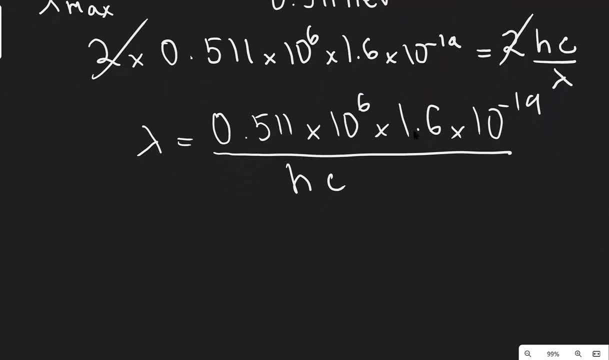 Lambda is 0.511. Times 10 to the power of 6. Times the electron charge Divided by hc. Now let's plug in some values. That h is Planck's constant, just 6.63. Times 10 to the power of. 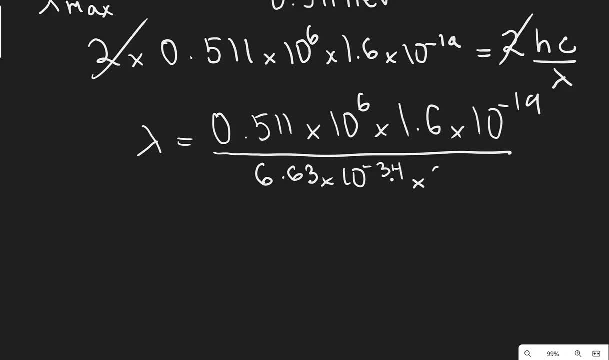 Minus 34 joules seconds. Multiply by the speed of light, Which is 3.0. Times 10, to the power of 8. Meters per second, And this here is of course The maximum wavelength. Plugging those numbers, 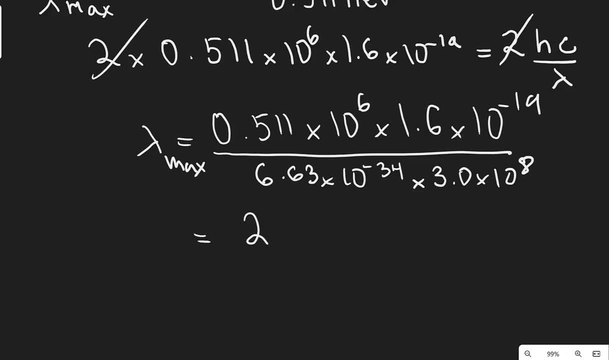 Into a calculator, We're going to get a number Around 2.43.. So 2.43.. Multiplied by 10, to the power of Minus 12 meters, Up to 3 significant figures For the maximum wavelength. 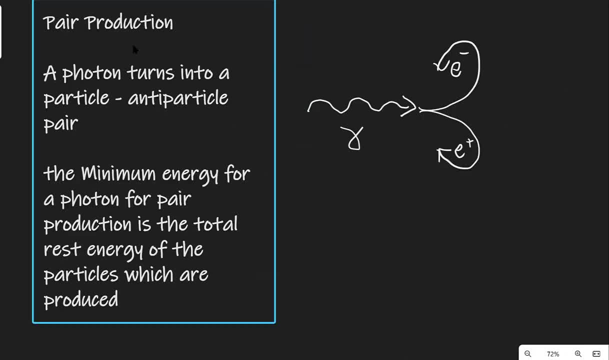 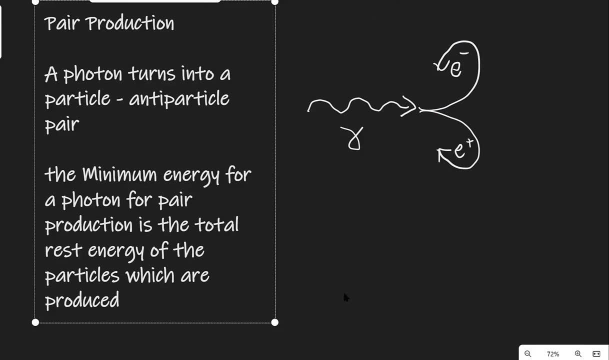 The opposite of Annihilation is known as Pair production. Now, in annihilation, We had two particles meeting up And producing photons. In pair production We have a photon Which turns Into a Particle antiparticle pair. Isn't the world of particle physics? 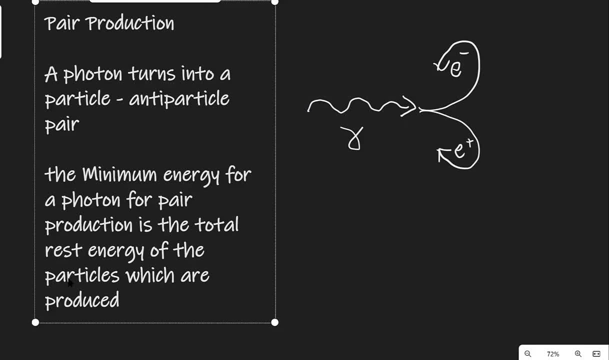 Strange and great. We just have this particle of light Which is just spontaneously turning into A particle antiparticle pair. Now the minimum energy for this to happen? Is that the energy Of the photon, Or the minimum energy of the photon? 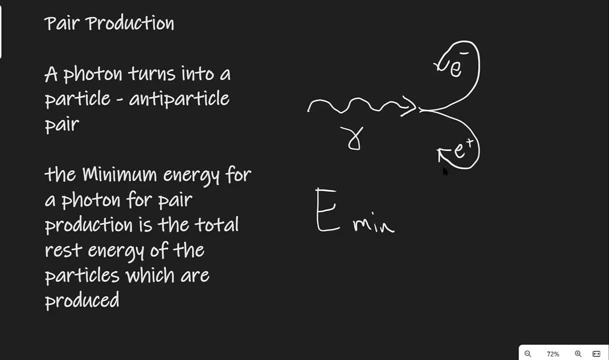 Which, once again, is given by HF or HT over lambda. That has to be Equal to at least Twice the Rest energy Of the particles. This is typically given by E naught, by the way. So we can say that E min is equal to twice. 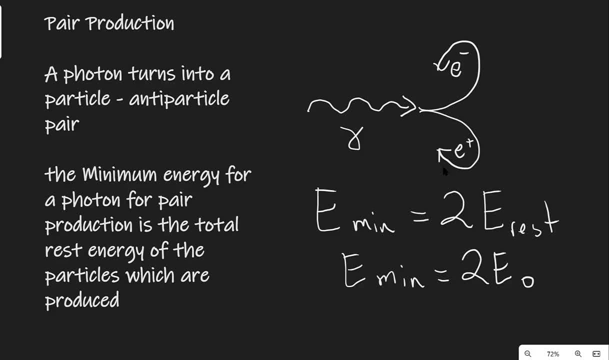 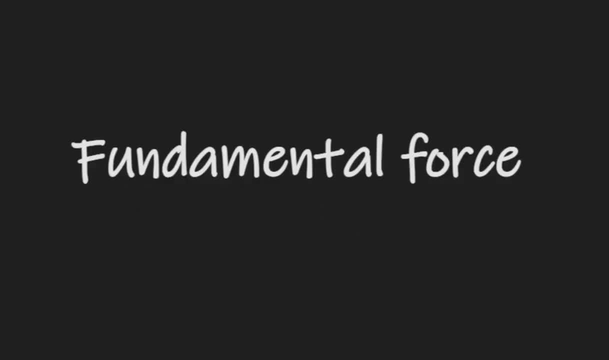 E naught For calculations. we can also, of course, use that E min will be HF or HC over lambda. Let's talk about what a fundamental force is. Most of the forces That you'll be familiar with Are not actually fundamental forces. 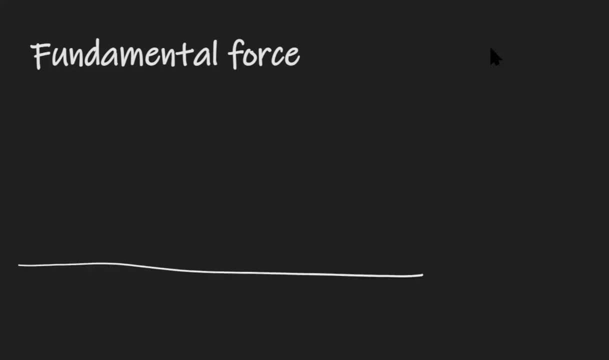 So let's take an example. We'll just say friction. So imagine that we have something like a ball Which is rolling with a certain speed, v. This speed will be continuously Decreasing due to a Frictional force Acting in the opposite direction of the movement. 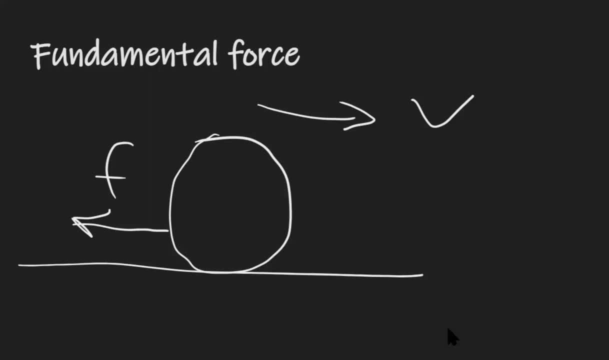 And what actually causes this force? Fundamentally, This force is actually an electrostatic Repulsion force. The surface of the ball Is not perfectly smooth. There will be some electrons Right on the outside And some electrons Right over here. 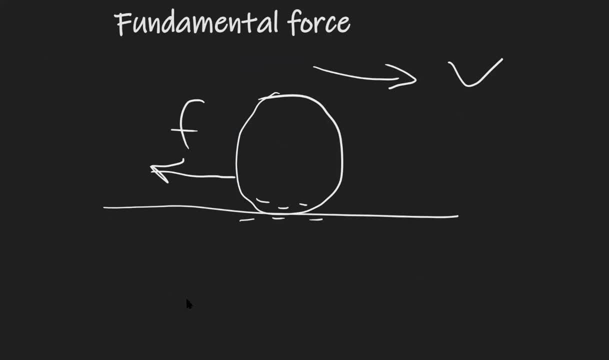 And this is ultimately an electrostatic force, Because the overall force Can be broken down to the individual repulsion By those electrons, Those electrons, Those electrons And those electrons all added up. Now, if we were to try and break down forces, 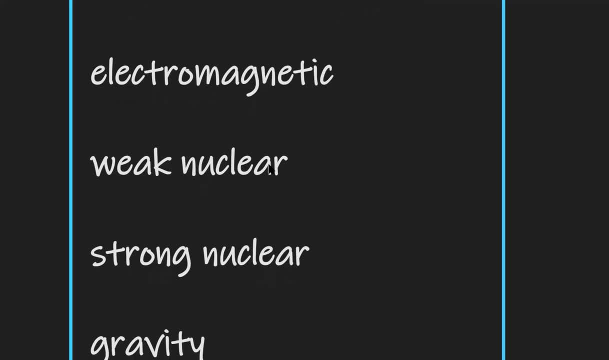 Further and further. There are only four fundamental forces: The electromagnetic force. The weak nuclear force That's responsible for nuclear decay. The strong nuclear force Which we talked about in the beginning of this video. This holds the nucleus together. So let's say: 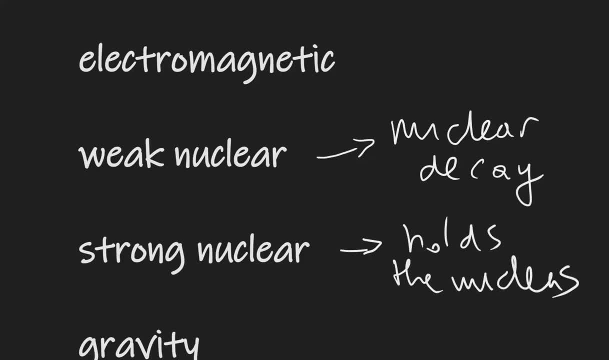 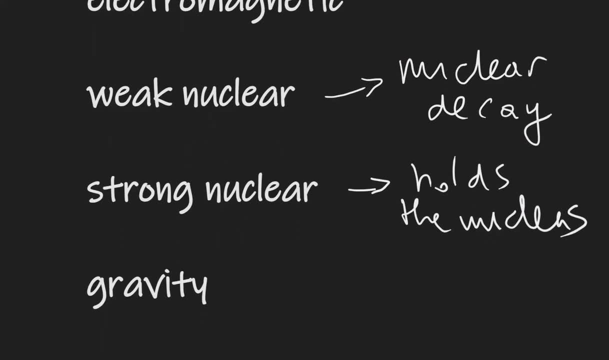 It holds the nucleus together. And of course We also have gravity. Now, gravity is considerably weaker Than the other three interactions And we tend to ignore that In particle physics Relatively often. We still don't have a Quantum gravitational theory. 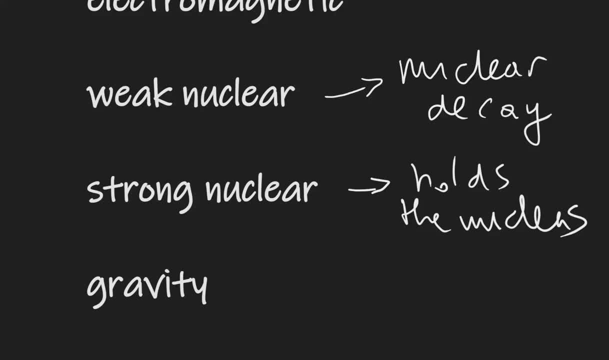 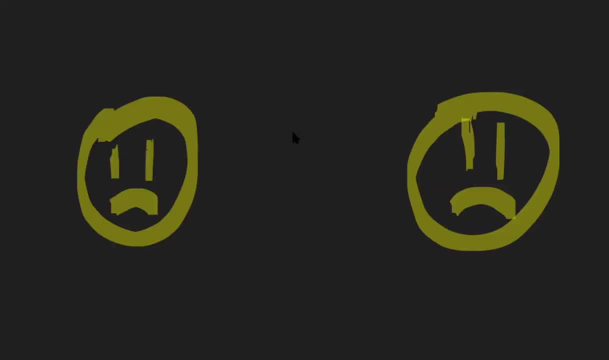 Or a quantum theory, Which is one of the holy grails Of physics That some of the brightest minds in the world Are actually working on. Here are two electrons. We can see that they are negative. What do the two electrons do? 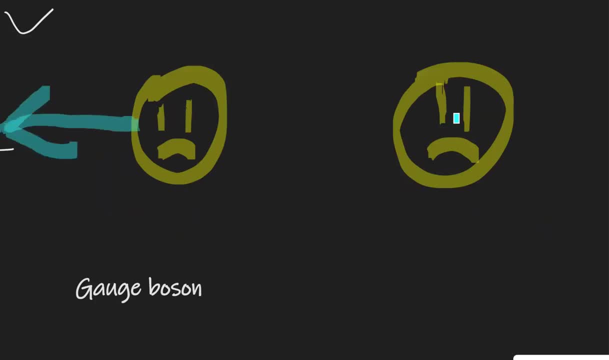 Well, they actually repel. So this means that there is going to be a repulsive force Acting in this direction On this electron And there is going to be exactly the same But opposite repulsive force Acting on the other electron. 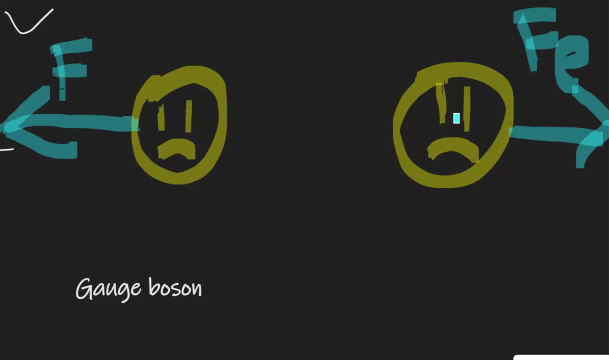 How do the two electrons know One another? Well, it turns out that the interaction Is actually carried by a particle Which is being emitted And exchanged by the two electrons. Change of a particle, Which is known as a Virtual photon. 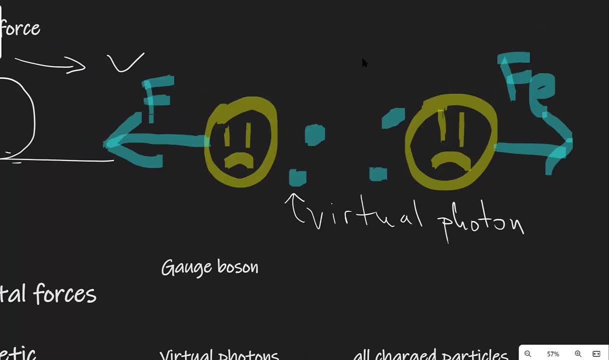 And actually The electromagnetic interaction Is carried out by this virtual photon. Now an exchange particle For any interaction Is known as a gauge boson. So should we just say over here: This is just an example Of an exchange particle. 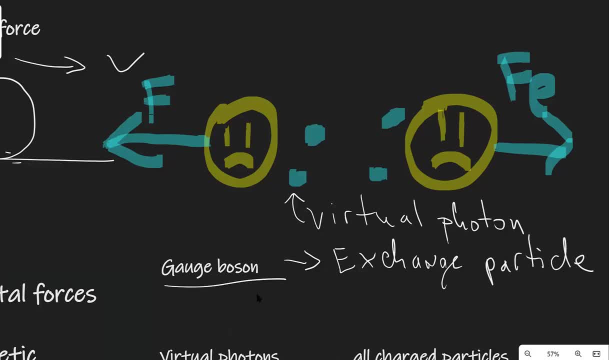 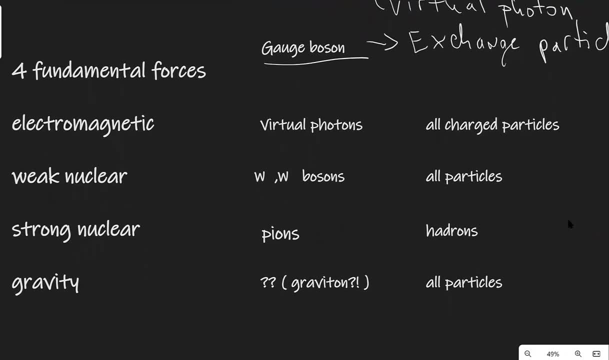 And they are different. For the interactions that we know, And I have listed them down here, So let's have a look. So, as we said, for the electromagnetic interaction, The exchange particle, Or the gauge boson, Is a virtual photon. 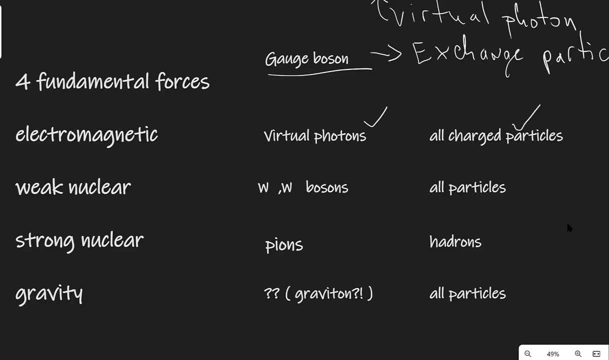 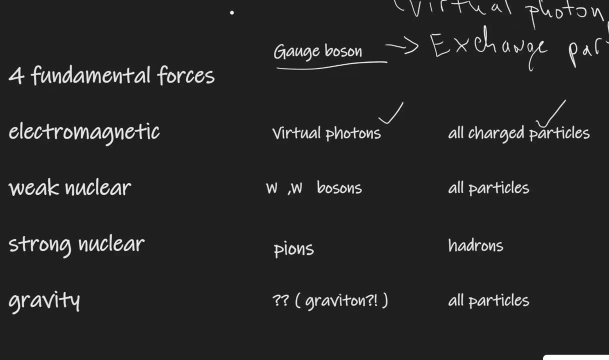 And the EM interaction Will affect all charged particles. Those are the weak nuclear force Which is responsible For nuclear decay. So the exchange particles There are W plus And W minus bosons. This can affect all particles, The strong nuclear force. 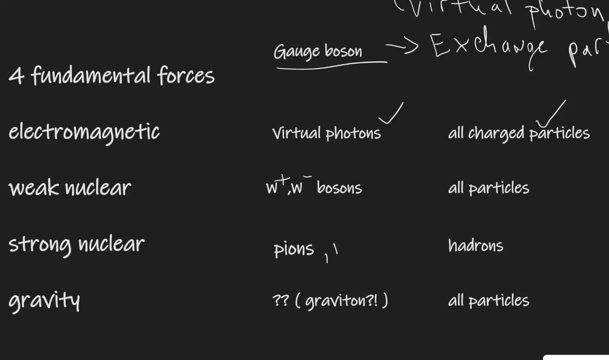 Is exchanged via the pions, Which could be the three types, actually Pi plus, Pi minus, Depending on their composition. There is also the pi zero particle. The strong nuclear force, importantly, Will affect only hadrons, Particles that Are only made up of 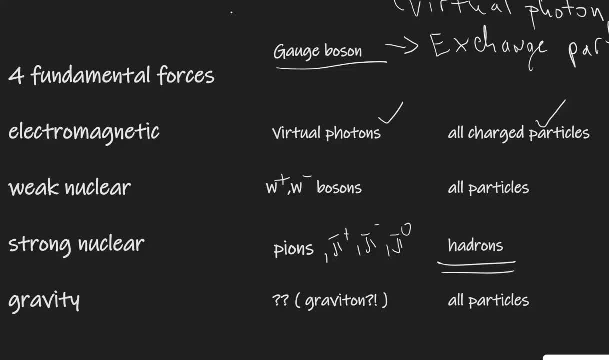 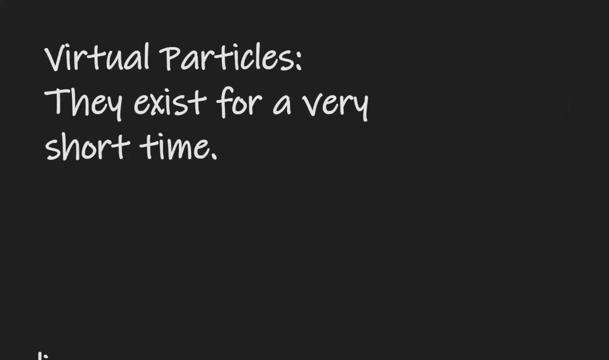 Works such as the proton Or the neutron, The fourth fundamental force In our list, Gravity. We don't yet have an exchange particle for it. There is a hypothesis About the particle known as the graviton, Talking about gauge bosons, by the way. 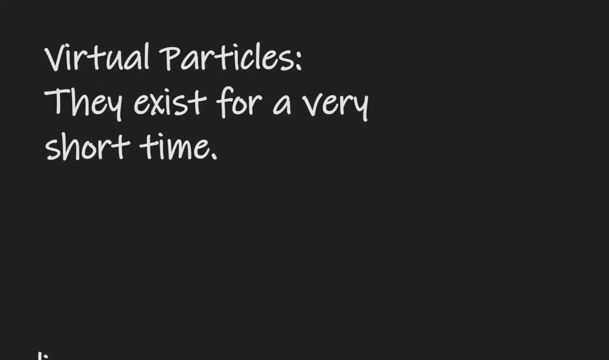 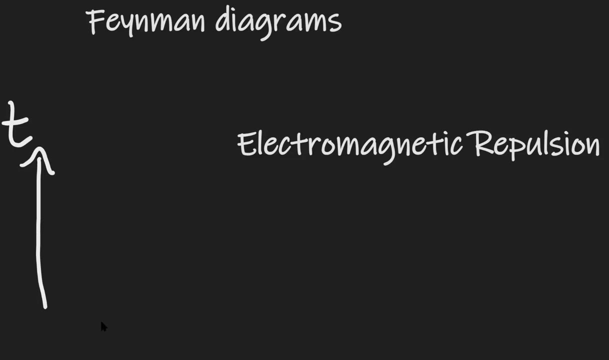 Lots of students often ask me: What are virtual particles? The answer is that they are real particles, Really, that exist For a very short time. And on to Refinement diagrams. next, The trick is to always Think about the y direction. 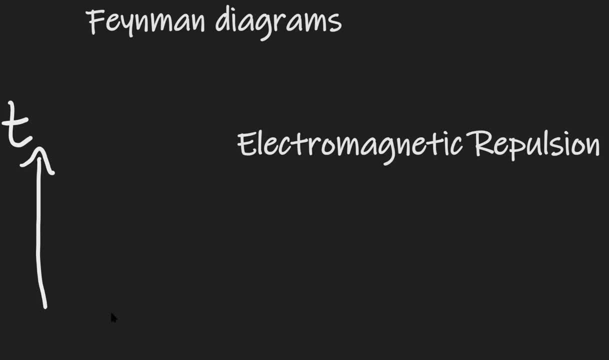 As time. What is actually physically happening to the particles? Let me give you a simple example, Looking at electromagnetic repulsion. So we are going to start off With a couple of particles Which are going to be repelling each other. So should we just choose two electrons? 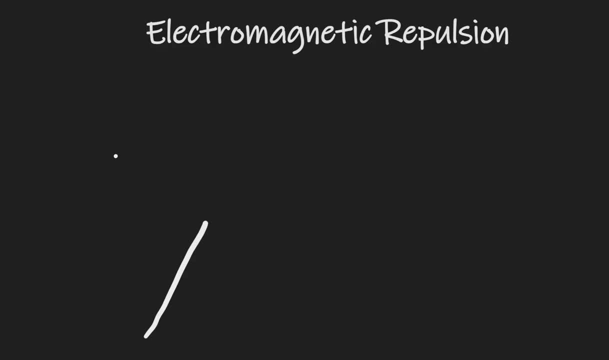 Represented by straight lines Kind of like this: And this is one electron, Let's label this as E minus This way, And we are also going to have another electron, Which is just up here, Which is E minus. As I said, the two particles are going to repel each other. 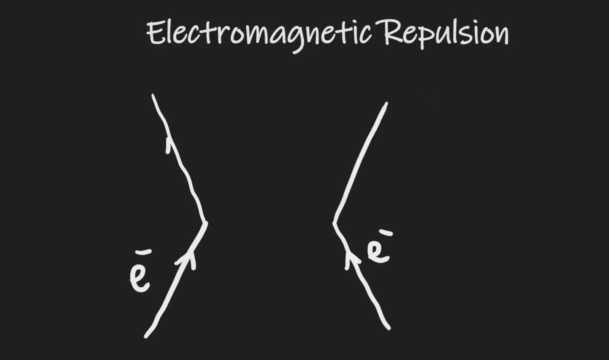 And we can represent this, like so And like so. We can add in some directions And label the particles After this interaction as well. Something must have caused That repulsion, And what has actually caused it Is a gauge boson. 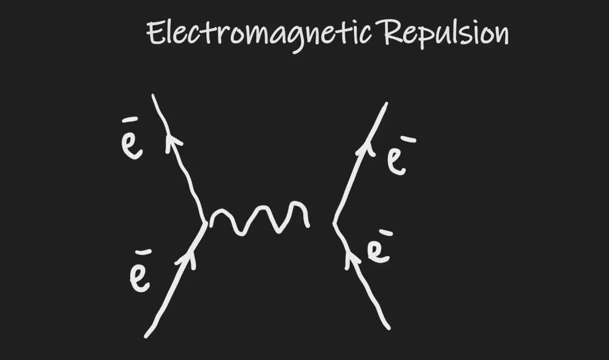 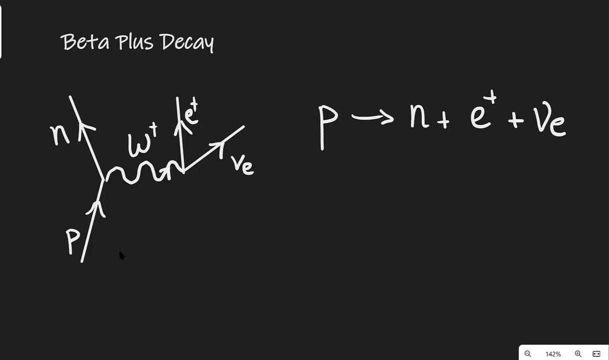 Which represent A squiggly line, And this is indeed Just a virtual photon. This is our first Feynman diagram. Another diagram That we need to know Is that of beta plus decay. In this type of decay, A proton will turn into a neutron. 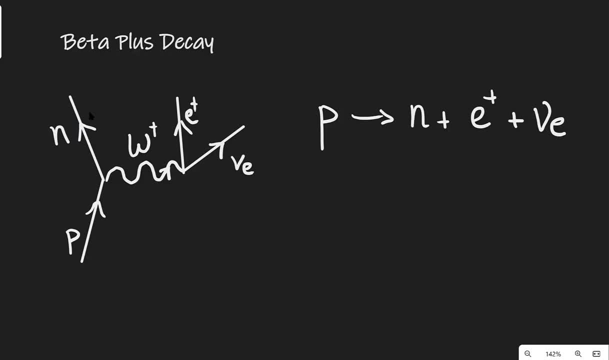 This happens When the quarks Inside of the proton Actually release a W plus boson And subsequently The W plus boson Will turn into a positron And a neutrino. The equation for this reaction Is that a proton 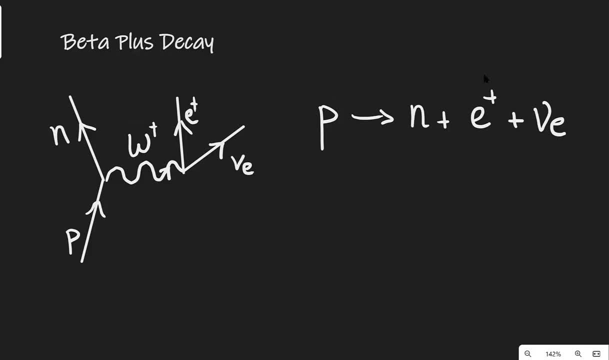 Will turn into a neutron Plus a positron Plus a neutrino. Notice how charge Is balanced in this reaction. For instance, the overall charge On the left hand side is one. The neutron has no charge. However, the positron has a positive charge. 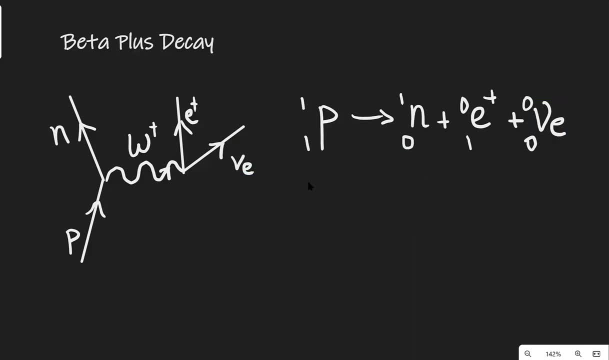 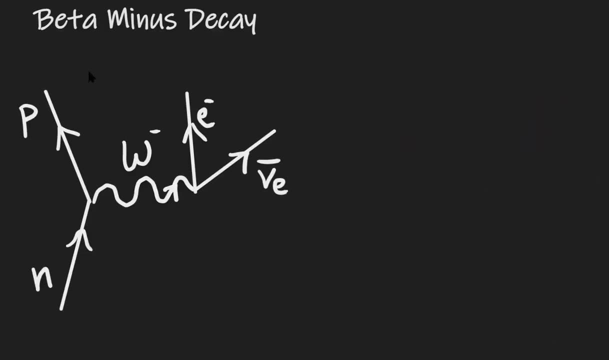 And the neutrino has no charge. So all the numbers On the left and on the right, Top and bottom, Are fully balanced. And here is beta minus decay. A neutron can turn into a proton With the release Of a W minus boson. 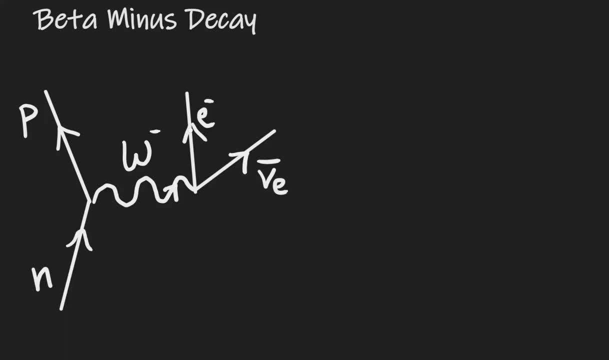 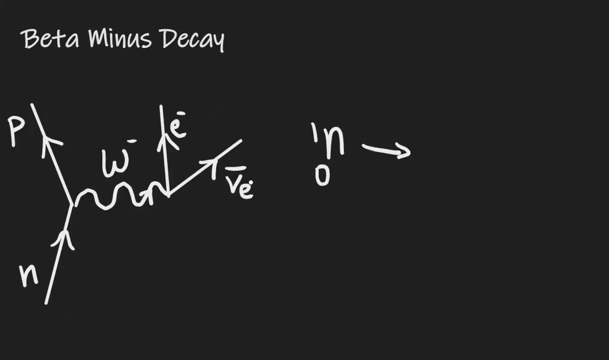 Which will then Turn into an electron And an anti neutrino pair. What would the equation For this reaction be? We are starting off with a neutron. The neutron is, of course, Zero one. This will turn into A proton. 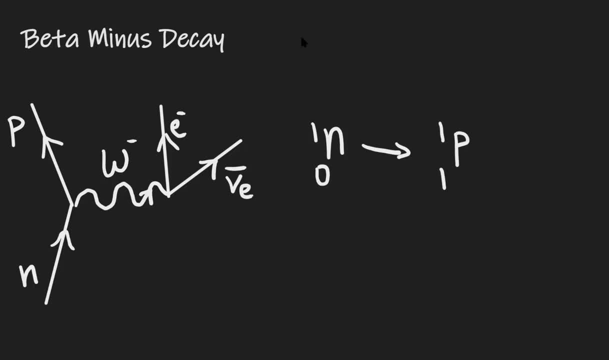 Which is just one one. And now we have a little bit of a problem Because on the left hand side The overall charge is zero. On the right hand side, The overall charge is one. So we need to balance this out With the addition of this electron. 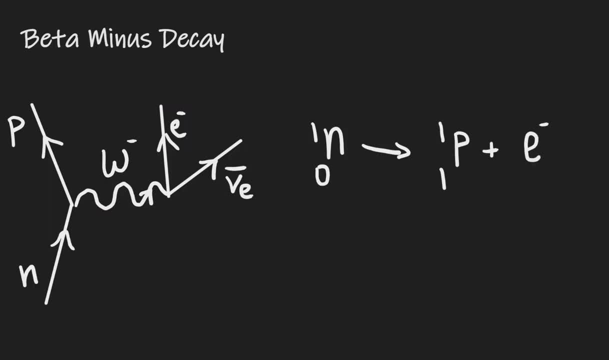 Over here. So we are going to have an electron, Which of course has a charge of Minus one. There is zero, the nucleon number. Then of course we are going to have The anti neutrino, Which is just zero, zero. 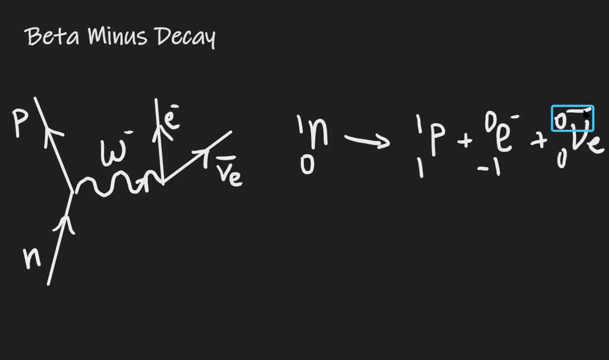 A good rule of thumb to remember, When this has the dash For the anti particles, That if you can see A negative sign within the electron, This means that we are dealing with A anti neutrino. One more Feynman diagram. 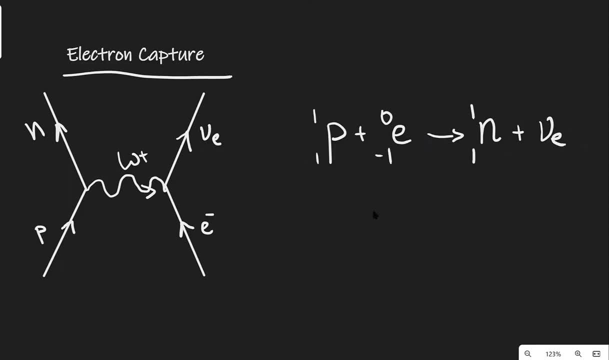 That we need to know about For the exam Is that of electron capture. In this diagram, We have a proton Which captures an electron, And the result is a neutron Plus an electron neutrino. Here is our proton And our electron. 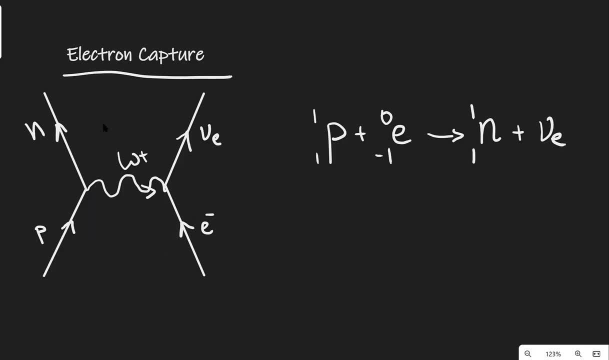 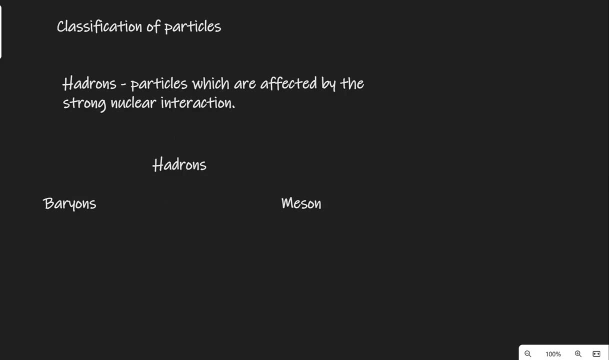 And as time passes, There is a release of W plus boson, And the proton turns into a neutron And we also have A neutrino left over. As particle physics progressed, We discovered Hundreds of thousands Of subatomic particles. 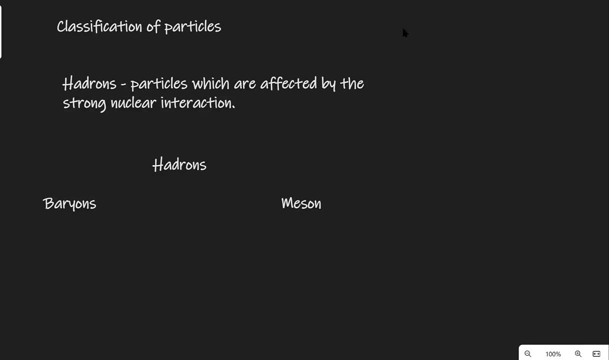 We needed a way To actually classify them Via the standard model. Let's have a look at some of the basic Terminology and classification of particles. First of all, we need to know That hadrons are particles Which are affected by the strong 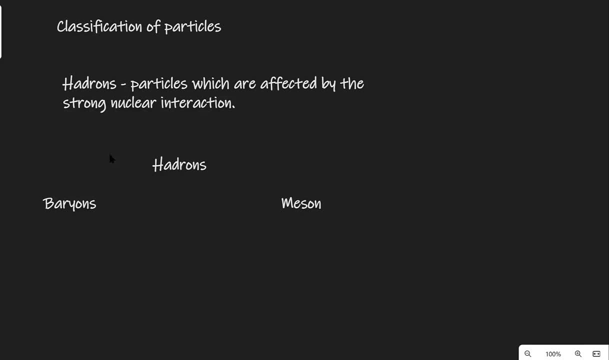 Nuclear interaction. They can be split into baryons. Now a baryon is just a hadron With three quarks And a meson. This typically has An example of a baryon: For instance, could be just the proton. 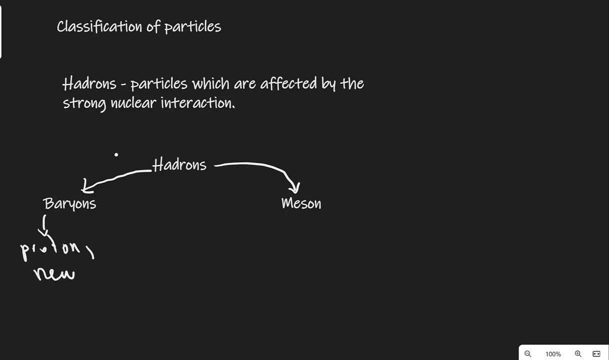 Could also be The neutron. A meson, On the other hand, Could be something like A pion, So we can just say That this here is a pion And we've talked about these, So it could be the pi plus. 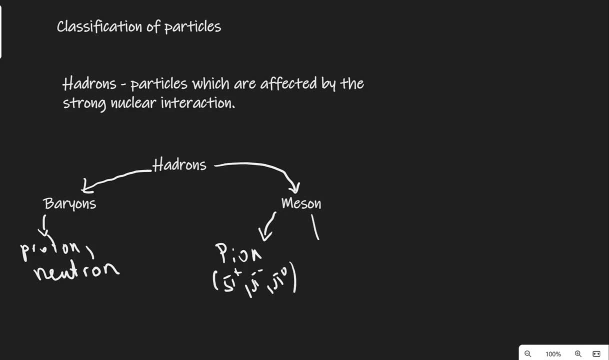 Pi minus The pi zero. And then we've talked about The other number called Kaons. There's quite a lot of them actually, And there's quite a few other mesons as well. The kaons as well Are pretty similar. 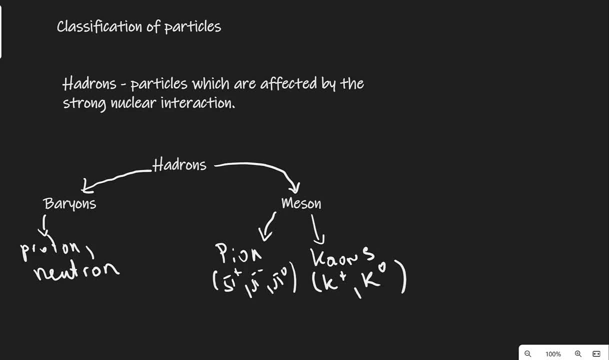 They have the k plus The k zero And quite a few others. It's important to note That particles can also Be described in terms of their Baryon number. This is another quantum number, B And for baryons. 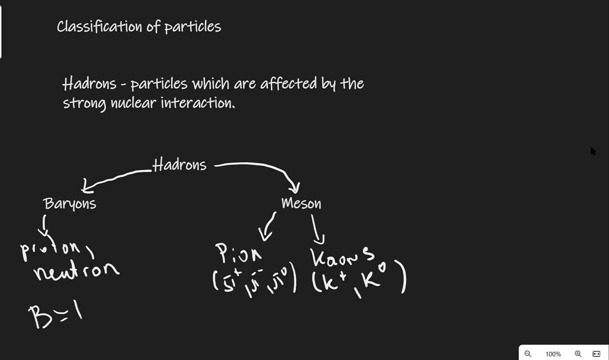 This is equal to one. So, those particles over here, They're gonna have a baryon number of one, Whereas for the mesons, Well, because they're not baryons, They're gonna have a baryon number of zero. 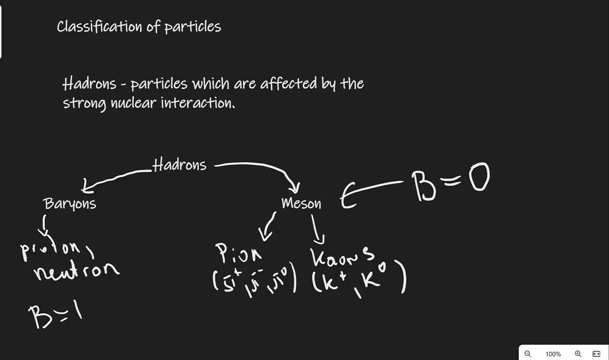 And this quantum number is conserved In a very similar way, in a reaction, Similar to the way charge is conserved. For instance, baryon number should be conserved. So if we start with one baryon, This could be a proton or a neutron. 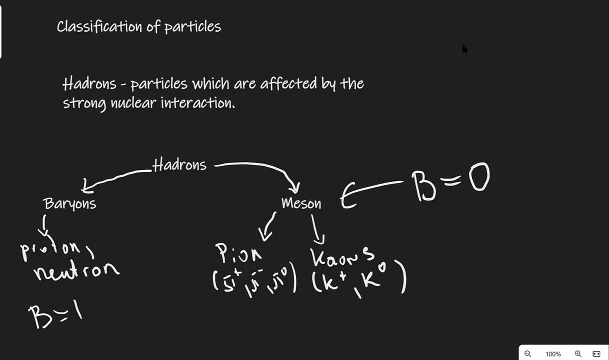 This is conserved. Baryons tend to be inherently unstable And, so far as we know, The proton Seems to be Actually the only stable baryon That we exhibit, Even though loads of experiments Are trying to find a proton decay. 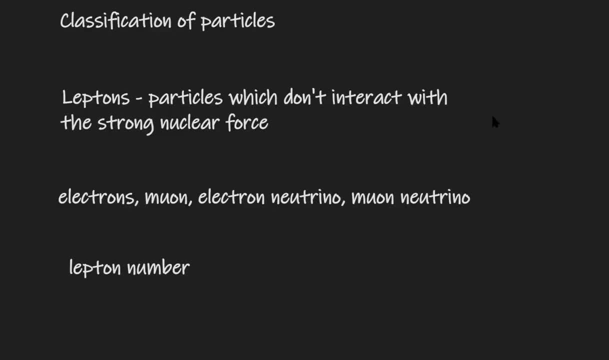 But so far this has been unsuccessful. Another major set of particles Are leptons. These are particles which don't interact With the strong nuclear force, For instance the electrons Or the anti electrons. The electron known as the positron Are examples of leptons. 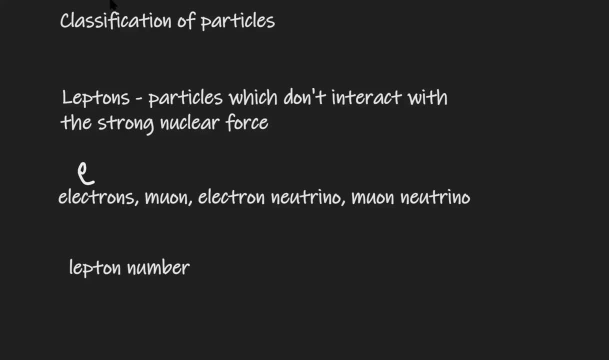 The muon. Should we just write their symbols here as well? So this is the symbol for the electron. This right here Is the symbol for the muon. So it's Just a particle like this. It's almost like the heavier cousin. 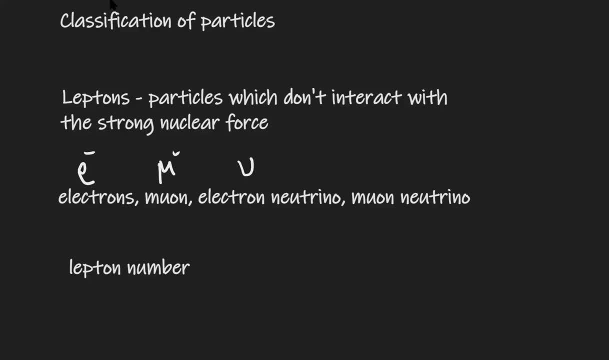 Of the electron. There's also the electron neutrino, Which is given like this, And we also have the Muon neutrino As the subscript of mu. Just like a baryon number, You can also conserve The lepton number. 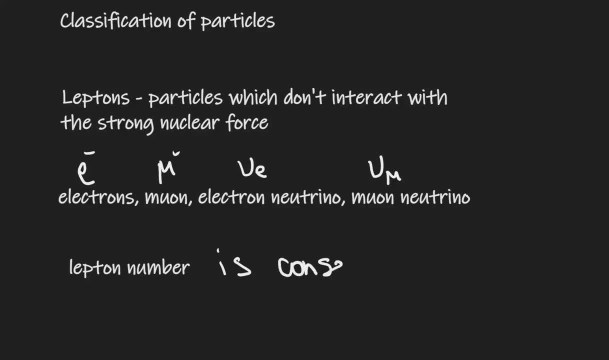 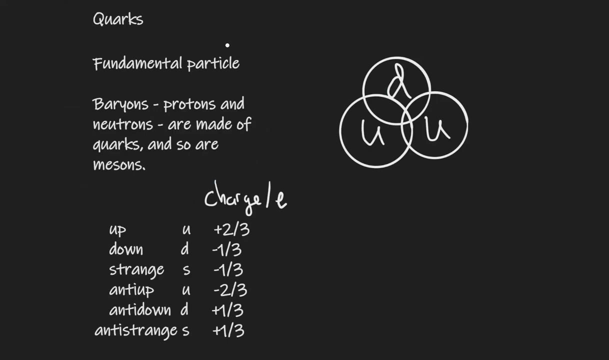 So we can just say that the lepton number Is actually conserved. The muon, though, Being a little bit heavier, Is unstable, And it will eventually decay To an electron. Now let's talk about quarks. They are a fundamental particle. 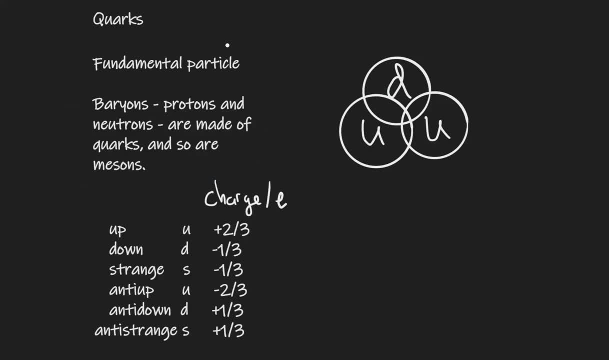 And baryons And mesons And hadrons Are made out of them. An example of this is the proton And also the neutron. They are all made out of quarks. Here are some of the properties Of some of the quarks that exist. 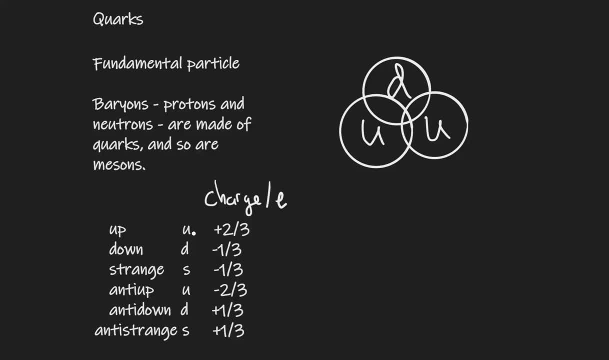 So, for instance, we have the up quark Which is labeled with a u And that has a fractional charge Of plus two thirds From the elementary charge. So that is plus two thirds e. The down quark Has a negative third. 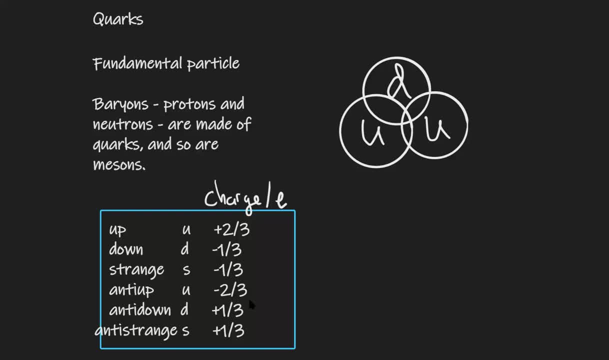 The anti up is negative two thirds, The anti down is just the opposite And the anti, strange- Has just the opposite. Now let me show you How the composition Of, let's say, a proton, For instance, is made Using the quarks. 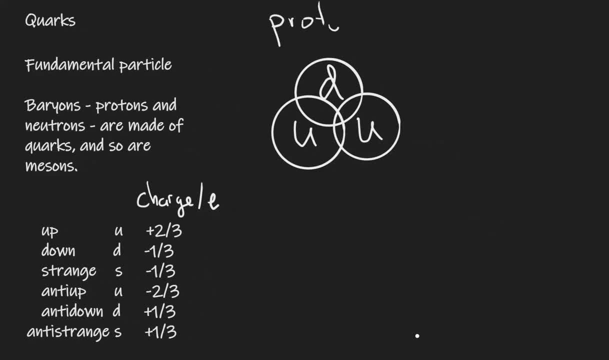 So this over here on the right hand side Is actually a proton And a proton, as you can see, Is just two u's And a d, And we can figure out the total charge. Let me just write the total charge On a proton. 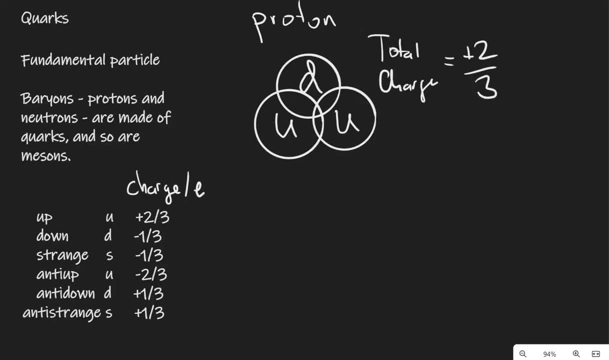 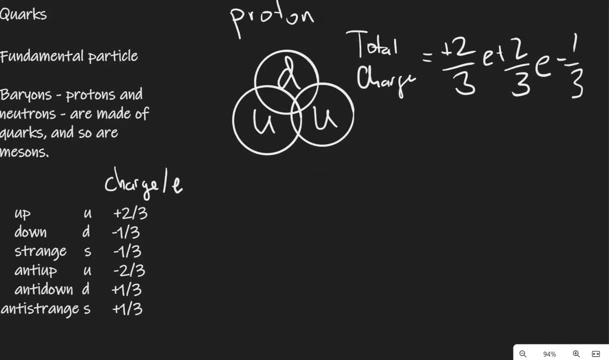 Now the charge of an up quark Is plus two thirds e, Plus two thirds e, And we also have a down quark Which is minus A third e. So this together is equal to Four thirds e. Take away a third e. 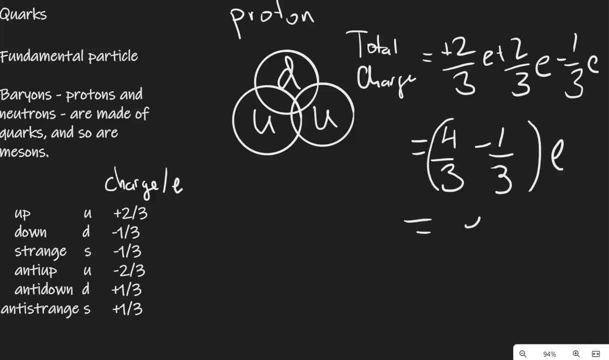 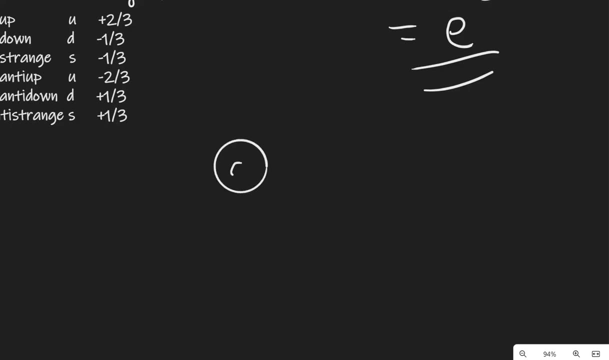 Which equals three thirds, Which is just e. So the charge On a proton Is well plus the Elementary charge, Let's do a neutron as well. So a neutron, on the other hand, Is made out of Two down quarks. 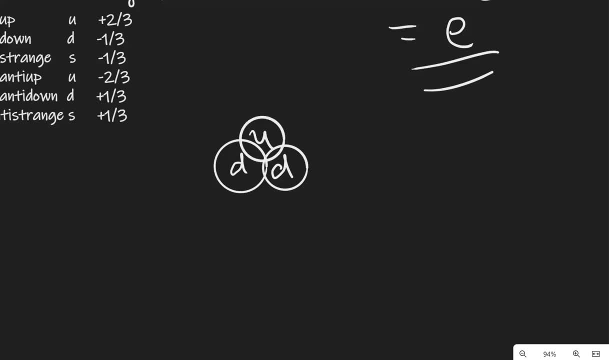 And also A? u quark. So two d's and a u. Now the total charge On the neutron Is going to be one up, Which is, let's just write: The charge on the neutron Is going to be equal to. 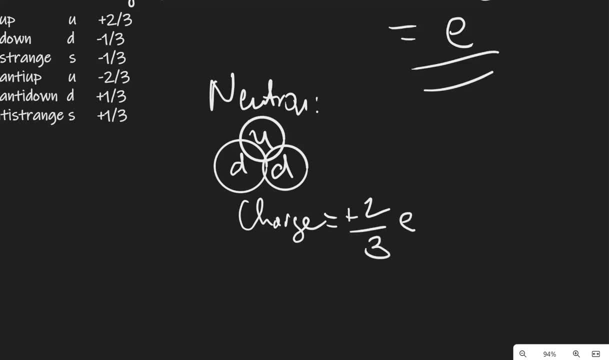 Plus two thirds e, And then we're going to take away A third e, And then we're going to take away A third e as well, And as we can see that this here Is equal to zero, It's important to know that the composition 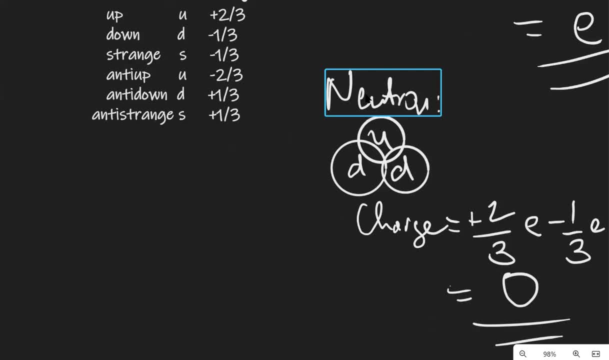 Of an antiparticle Such as the antiproton Or the antineutron. Should we just talk a little bit about the antineutron? It's going to have exactly the same composition But opposite, So it's going to be made. 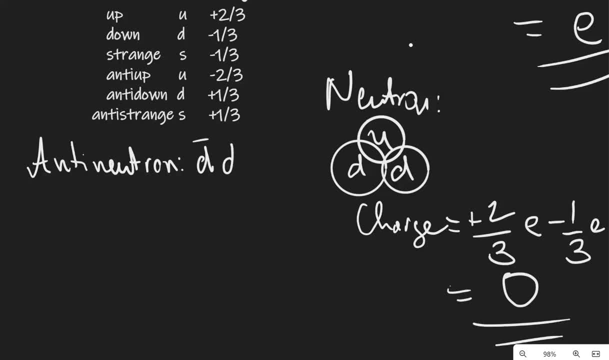 Out of two antidowns. Oops, we need to add some dashes over here To the antiparticles. It's going to be made out of Two antidowns And an antiup, And if we were to add up Those individual charges? 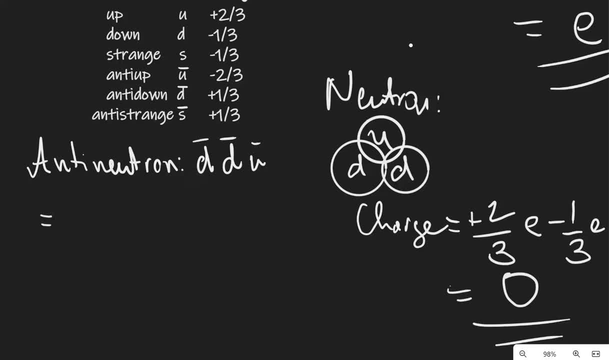 We're still going to get zero. So, for instance, the antineutron Will be made of two antidowns, as we said, Which is going to be plus a third, Plus a third, And then the antiup, Which is going to be minus. 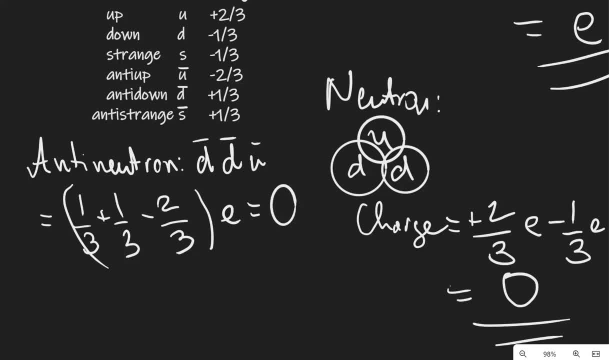 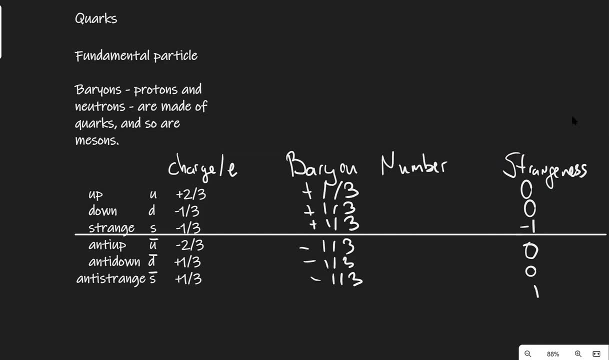 Two thirds, Which of course Is equal to zero. It's also important to note that in quarks There are two more quantum numbers That are conserved, So we're going to be conserving the baryon number And the strangeness. 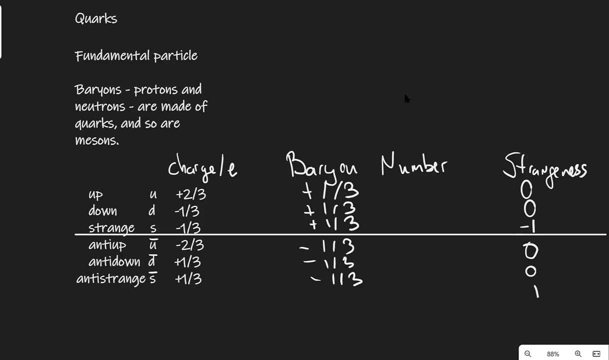 So the baryon number Is just a third, Which makes sense because it's three quarks To make a baryon. So the individual quark Is going to have a fractional baryon number Of plus a third. 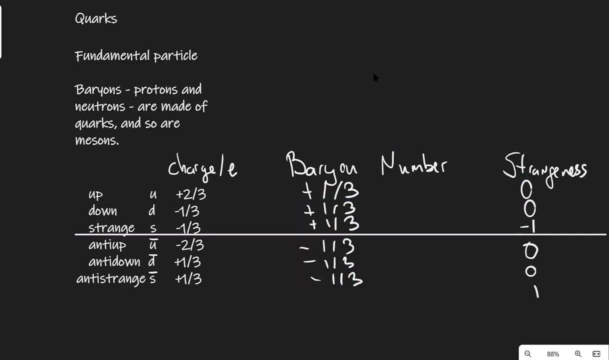 Plus a third for normal matter And minus a third For antimatter. There's another Strange quantum number, Known as strangeness, Which is zero, Unless we're talking about a strange quark. Now the strange quark Has a strangeness quantum number of minus one. 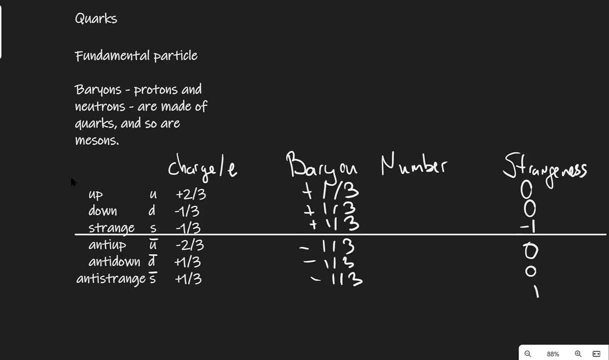 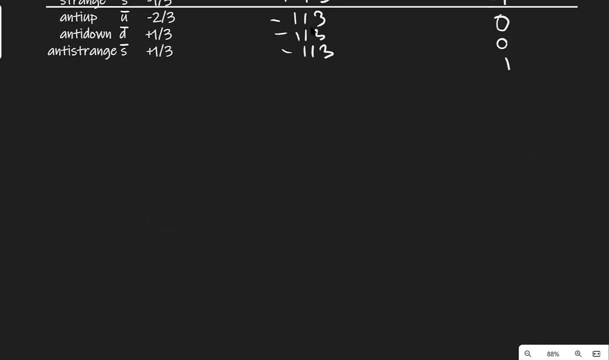 Which is super interesting. I'm going to show you a whole other video, And the anti-strange quark Has strangeness of one. Finally, let's talk about one more point of the spec, And that is the decay Of a neutron. 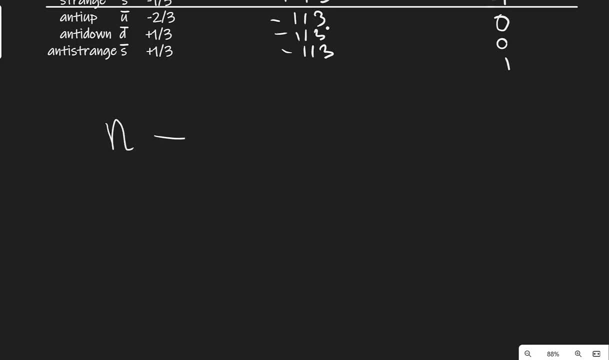 So this is just the standard beta decay, In which a neutron Turns into a proton. Now remember, the neutron Is one zero, The proton is just one one, Meaning that we're going to need an electron, So it's going to be minus one zero. 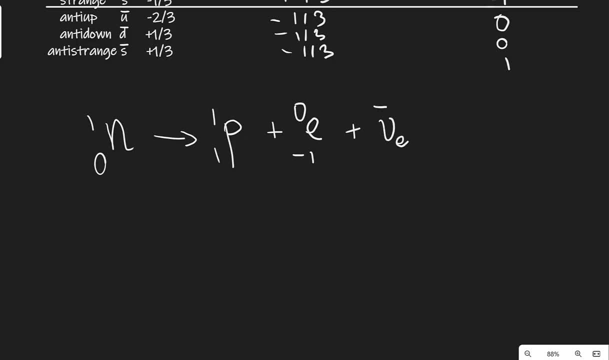 Then we also Have an anti-electron Neutrino. Well, if we think about the actual Composition of this, Because a neutron is Two D's And a U, And the proton is Two U's and a D-